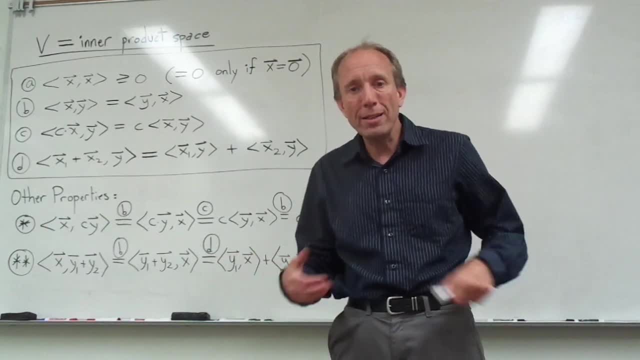 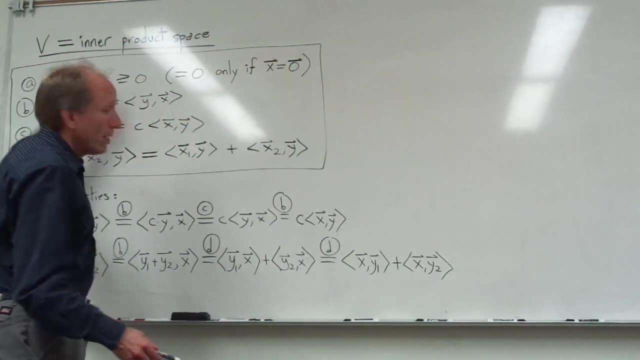 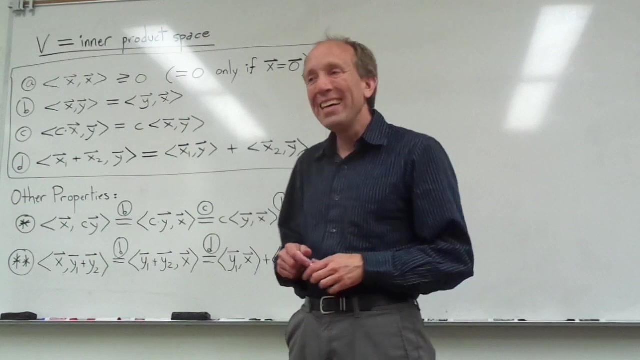 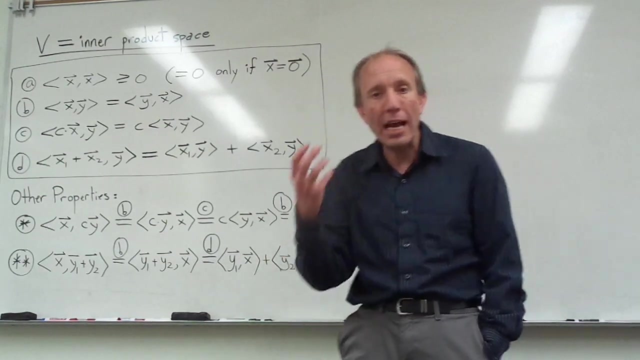 Remember that the whole idea of this inner product construction is that we're going to try to equip our vector space V with some geometry insights, with some geometric concepts, And to do that we have to have an inner product. An inner product on that vector space is really just an assignment of a number to every pair of vectors. 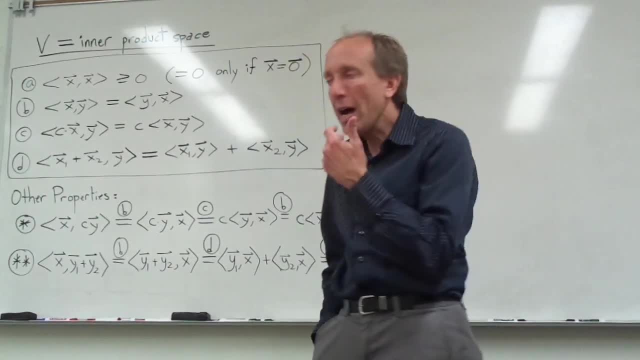 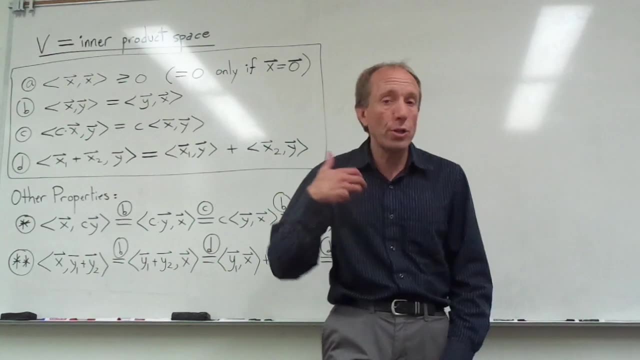 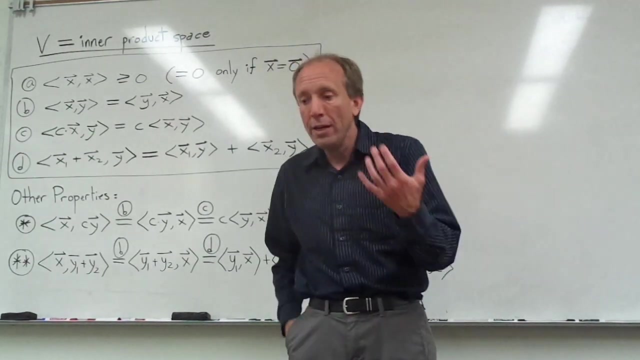 So if I take two vectors in my vector space, I can calculate their inner product by using an inner product formula that somebody is going to give us. It could be the regular dot product. if we're talking about vectors in Rn, It could just be the dot product that we've been familiar with from previous courses. 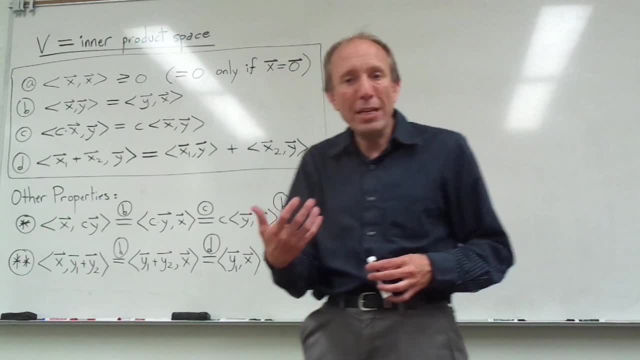 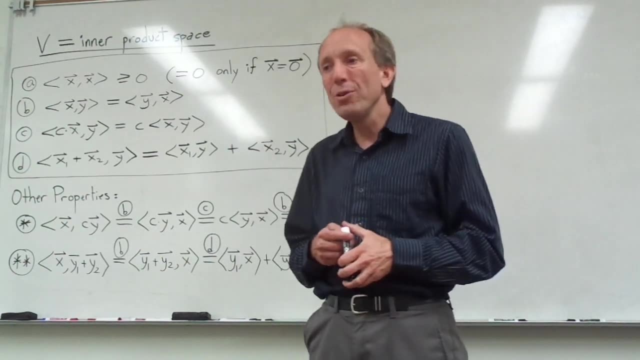 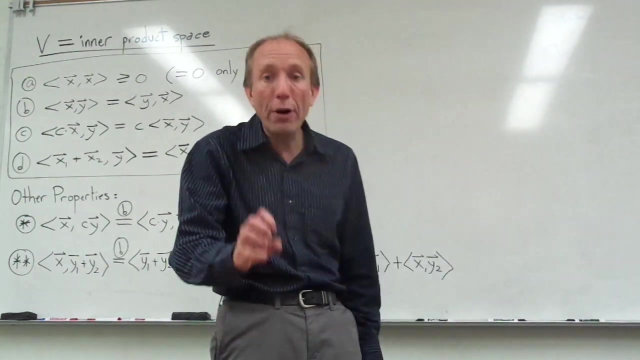 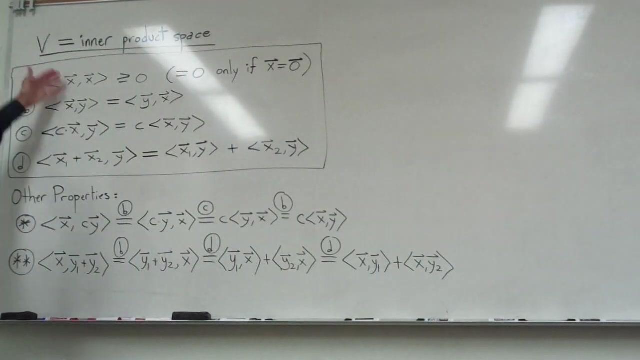 But it doesn't have to be that Our vectors might not be traditional vectors in Rn. They might have polynomials or functions or something like that, And so we have to be open to other ways of defining this inner product. However, no matter what our inner product is, no matter what our vectors look like, the inner product has to obey these four axioms- A, B, C and D- that I've put on the board. 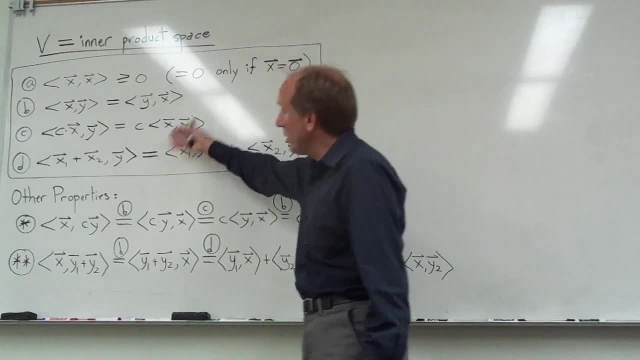 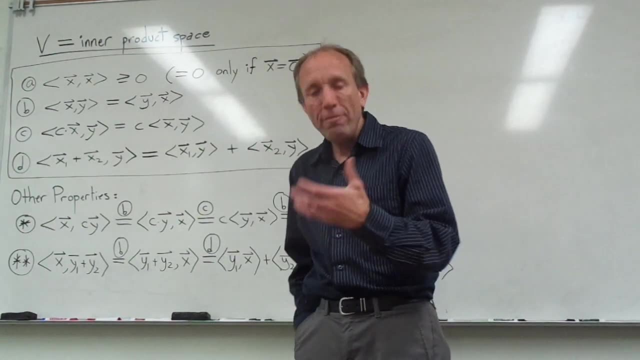 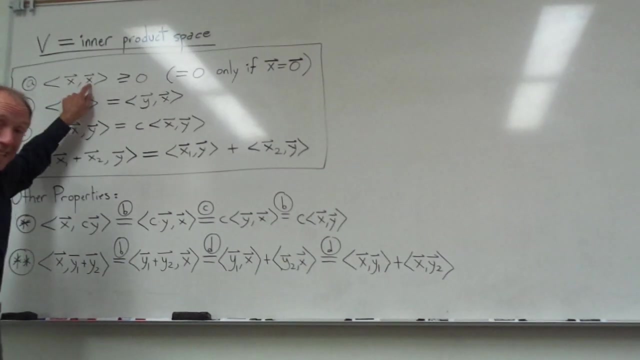 Okay, I already went through this list with you before. I just wanted to remind you again. When you take the inner product of two vectors, you're going to assign a number to that pair. If you choose to take the same vector twice, the number that you assign has to be at least zero. 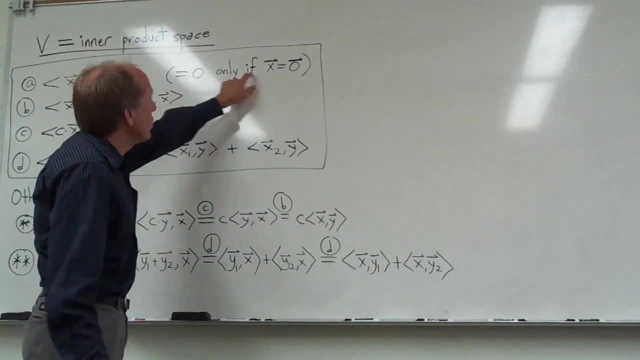 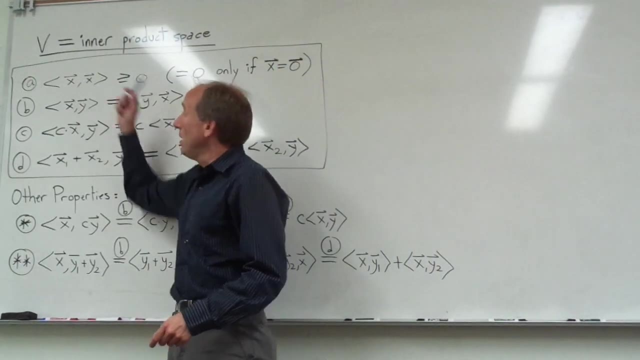 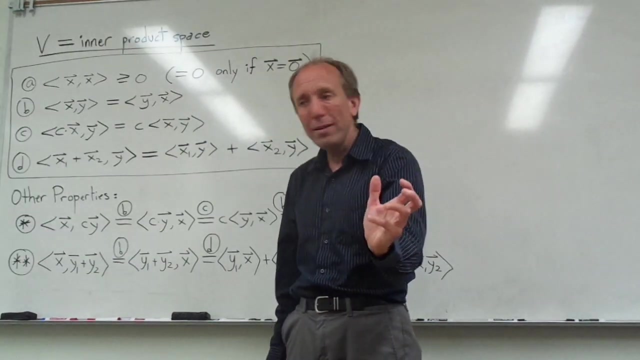 That's one of our requirements, And it can only be equal to zero for the zero vector itself. So for any non-zero vector, the inner product of the vector with itself has to be strictly positive. Okay, The order in which we take this pair, x and y, doesn't matter. 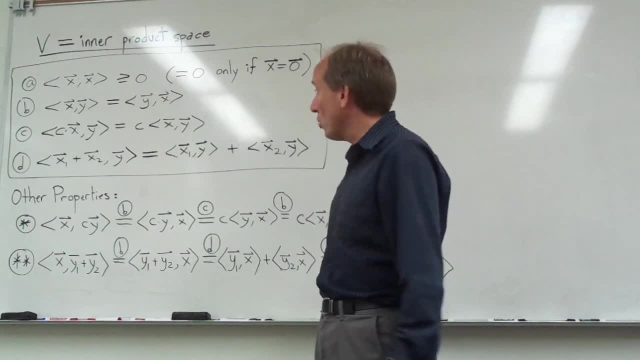 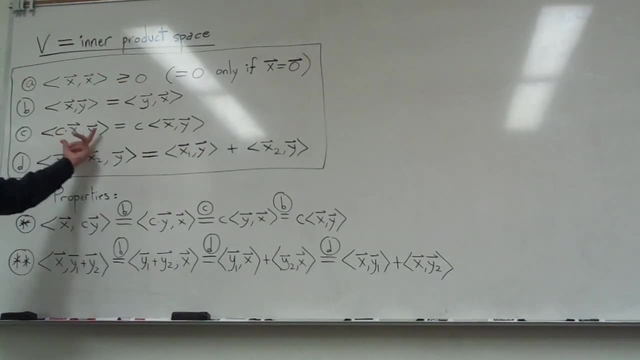 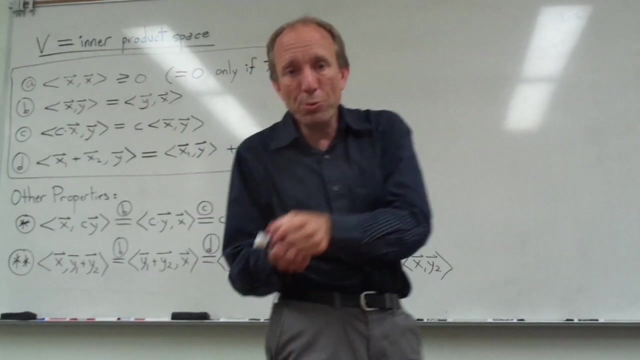 So I can switch the order. That's what condition B is requiring. Condition C tells me that I can factor constants out from the first vector in the pair, And condition D tells me that I can distribute a plus sign if it occurs within the first entry in the pair that you're taking the inner product of. 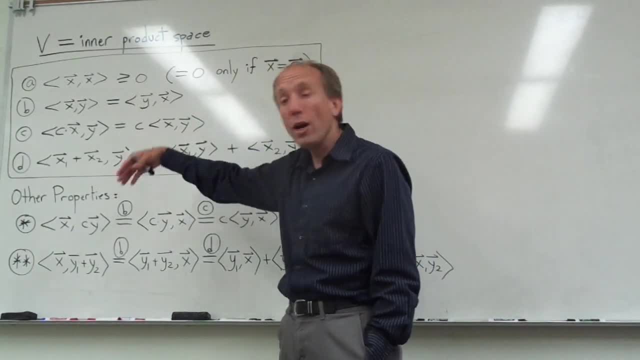 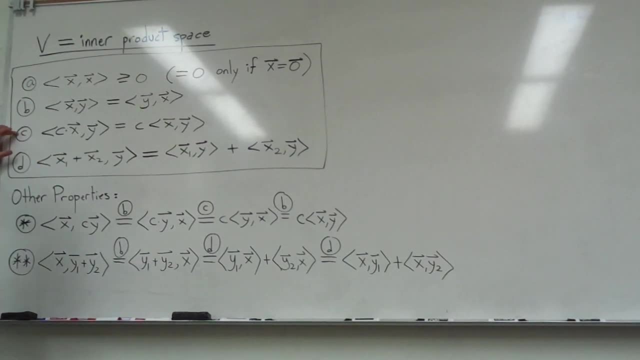 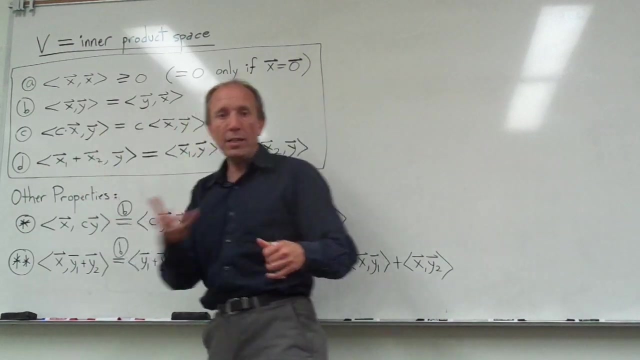 Okay, So these are the four axioms. Now there are other properties that you can now deduce from these axioms. For instance, both properties C and D also work with respect to the second vector in the pair, So I put these down here as star and double star. 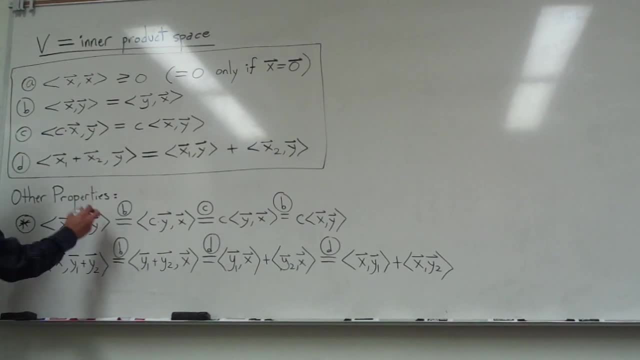 I can factor a constant. You look here at the beginning. I can factor a constant out from the second slot In the same way that I can factor a constant out from the first slot. And this is just the little proof that you can do that. 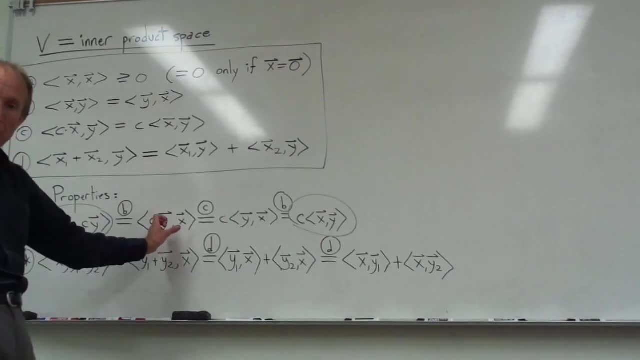 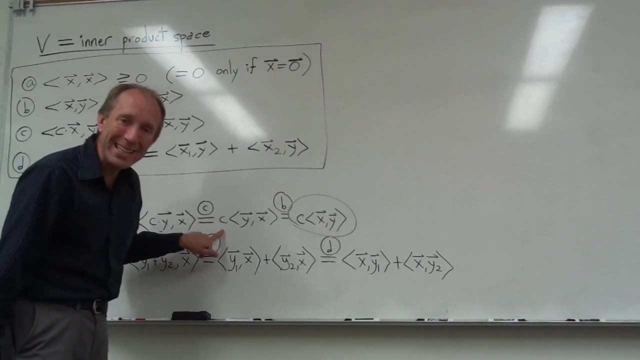 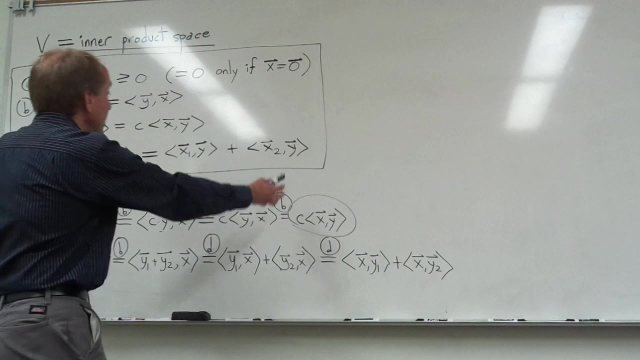 Essentially, you just switch the order of the two vectors by using property B, Then you pull the constant out by using property C, And then you switch the two vectors back again. Alright, So this is a new additional property above and beyond the axioms that we have in the list of properties. 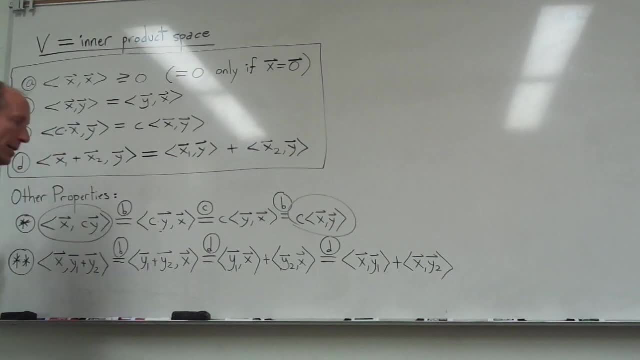 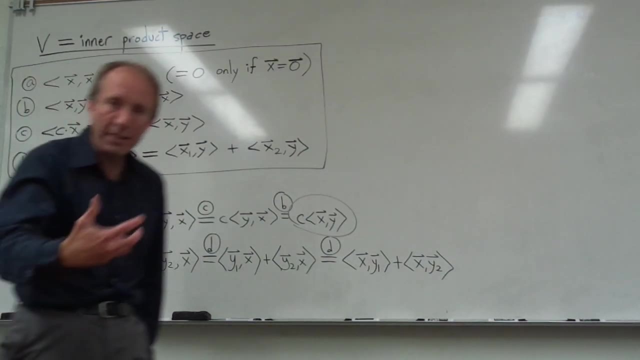 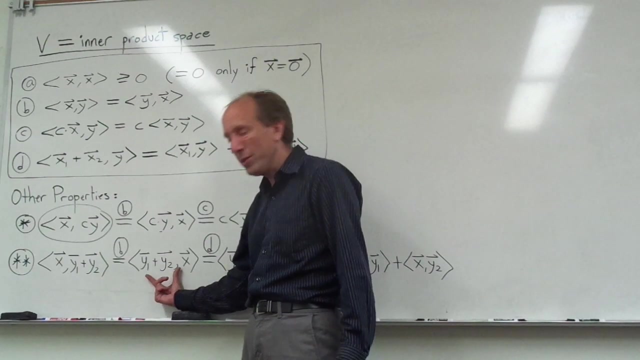 And the list in this box up here. Same thing for the fourth axiom. If I have two vectors added together as the second component of my pair right here, Well, I can first switch the order of the two components, Then I can use property D to split up the plus sign. 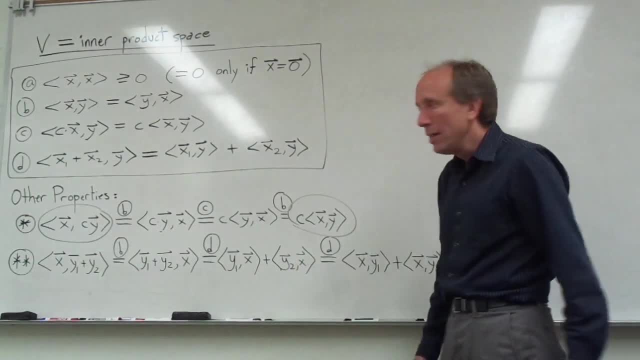 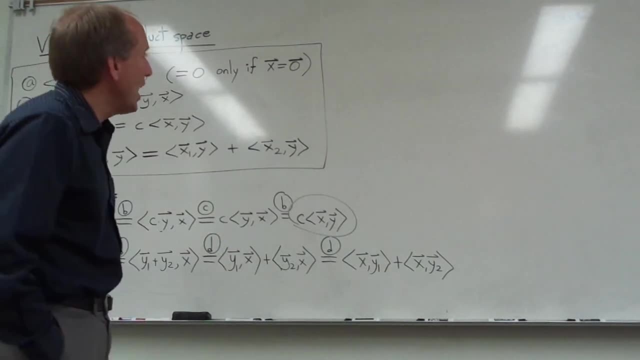 And then I can switch them both back again. So in that way, the C and the D, both of those properties, work in both the first and the second slot. Okay, Anyway, so we've seen a few examples of inner products already. 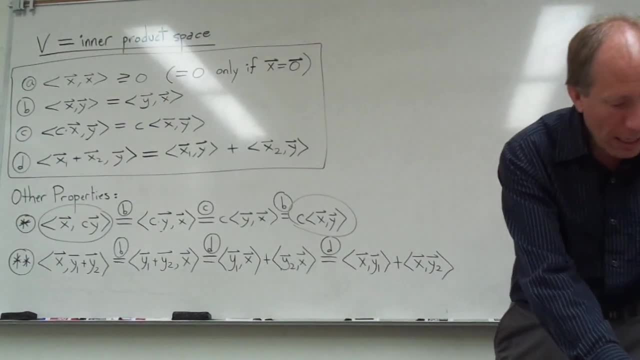 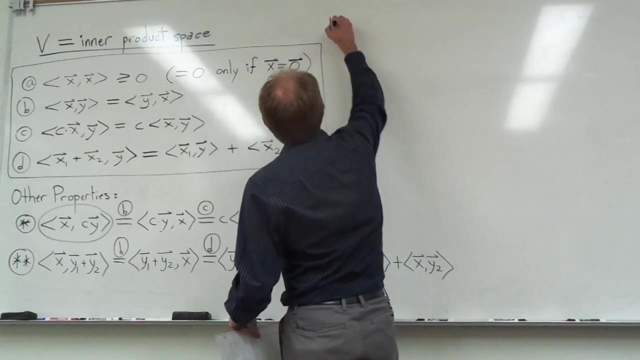 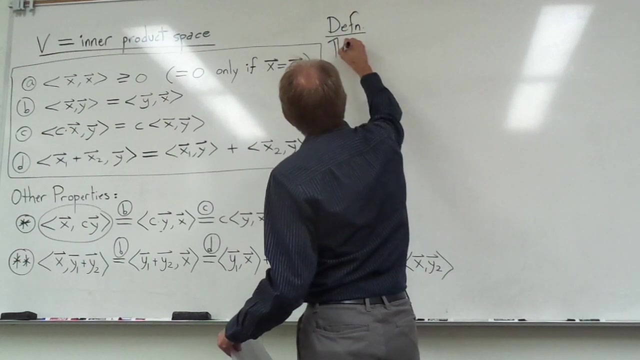 I want to give you just a couple more definitions here, Just to make sure that everybody's familiar with this material. This is pretty easy stuff. Let me just tell you about the length of a vector. So this is a definition here. You could say that the length 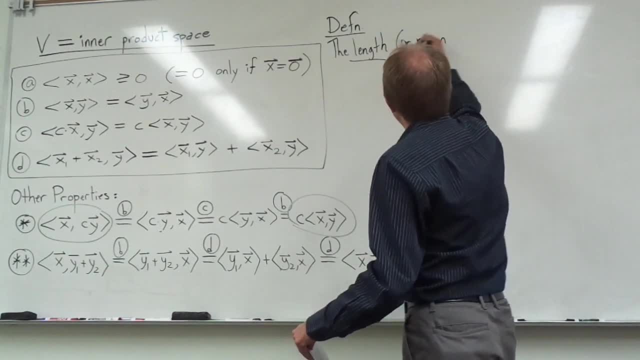 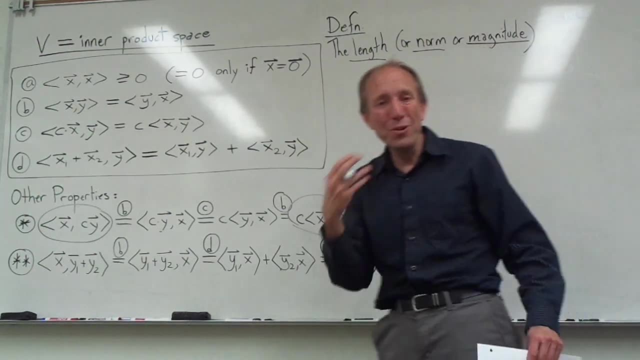 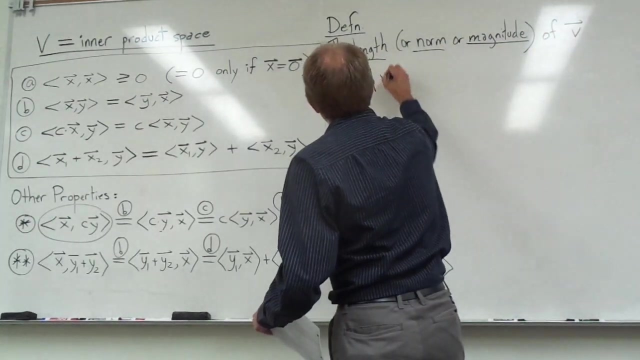 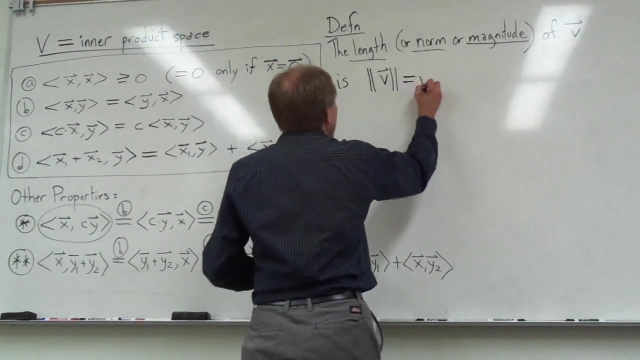 and that's also called the norm, And it's also called the magnitude. So the length or the norm or the magnitude of a vector V is. it's simply going to be. we use this double absolute value, bar notation for this, And the way it's calculated is: you take the square root of the norm. 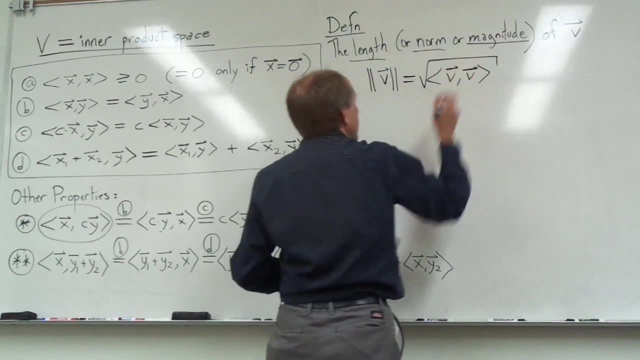 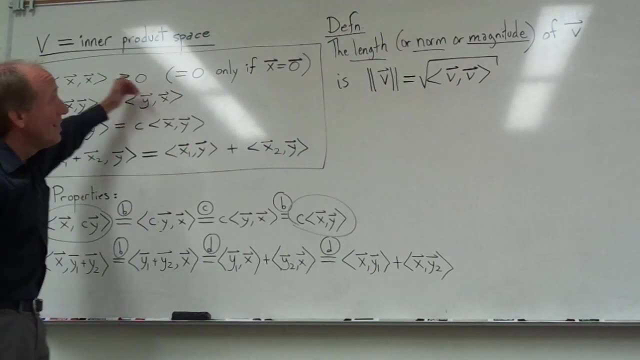 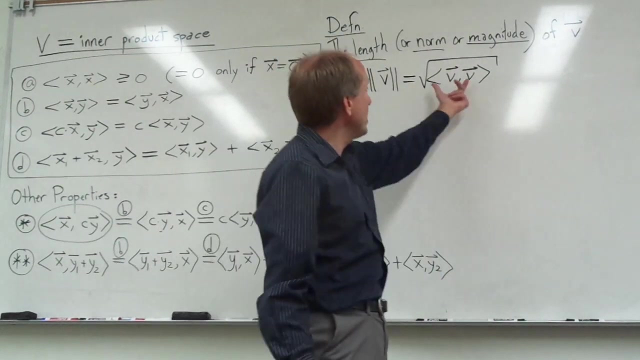 I'm sorry, the inner product of the vector with itself. Now notice that the inner product of a vector with itself is always at least zero. So that means that the norm of my vector- I can take the square root of this quantity, because what's underneath that radical- is always at least zero. 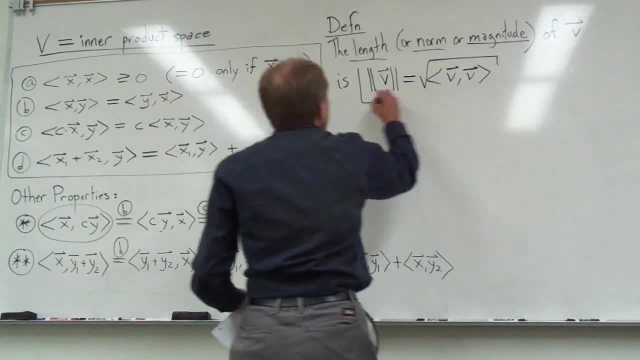 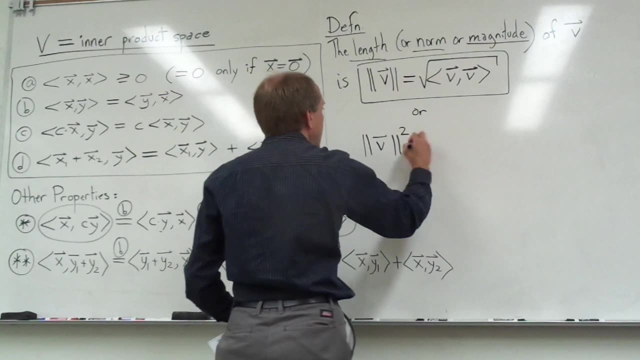 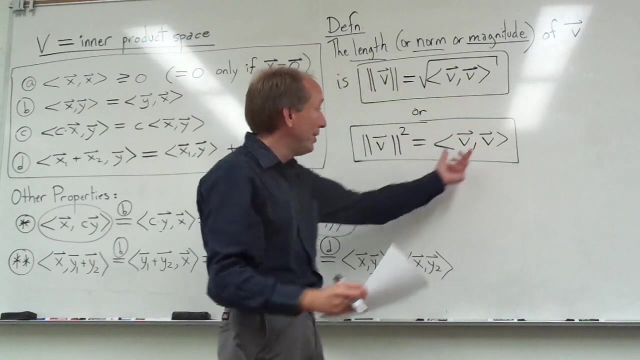 We're not taking the square root of a negative number here. So this is a very useful formula And it will sometimes be written. we will sometimes see the usefulness of just looking at it from this perspective, without the square root on it. So if I take the inner product of a vector with itself, 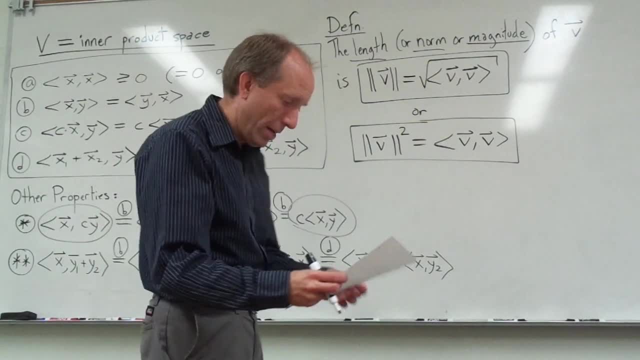 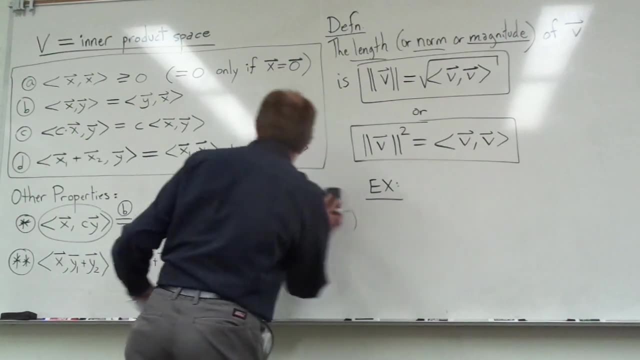 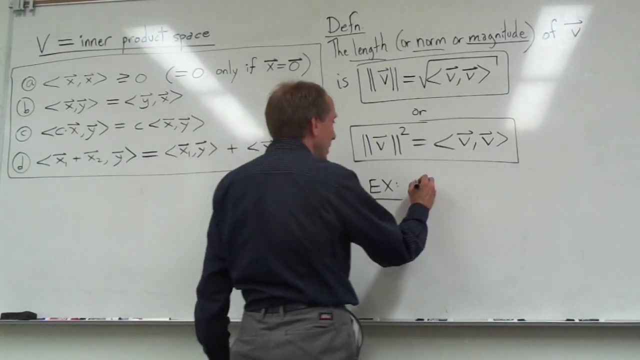 I get the norm squared of my vector. So for example- let's just do a quick example- I'm going to erase these properties here. Just want to show you a quick example of this. Let's suppose that I take you know. 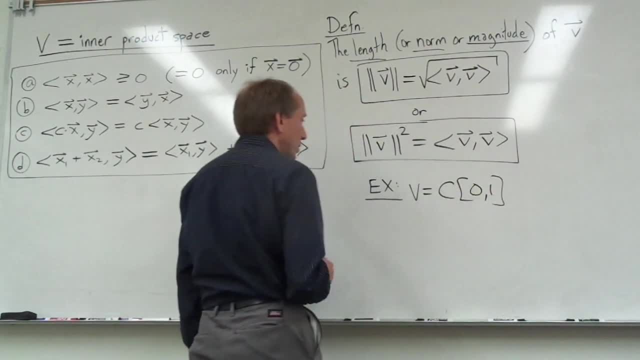 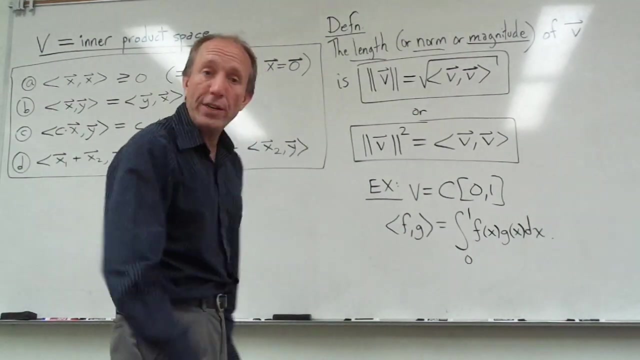 v to be c of, And I'm going to define my inner product in what is a fairly standard way: the integral from zero to one of f, of x, g, of x, dx. Let's figure out the norm of e to the x. 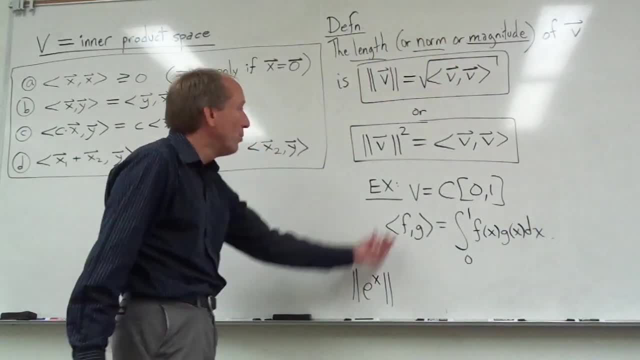 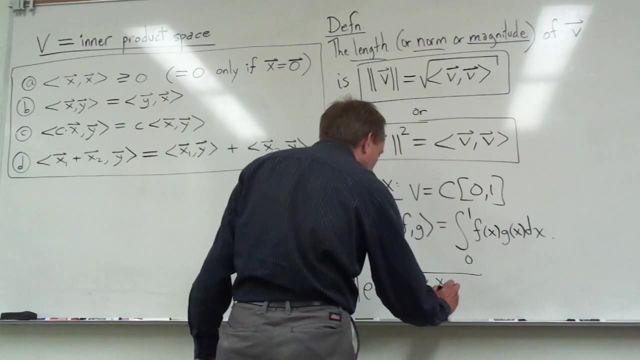 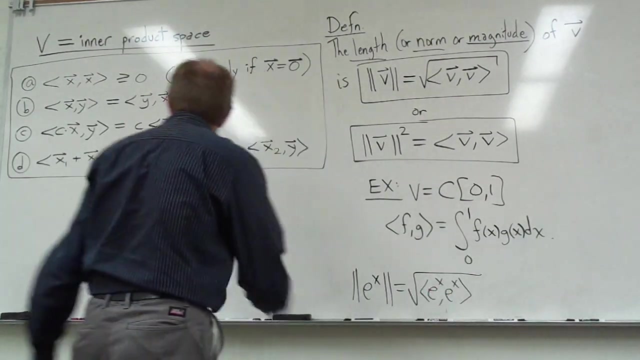 So the length of that vector within this vector space. So of course I have my formula: It's just the square root of the inner product of e to the x with itself. Okay, So I have to calculate that inner product. Now let me come back over here. 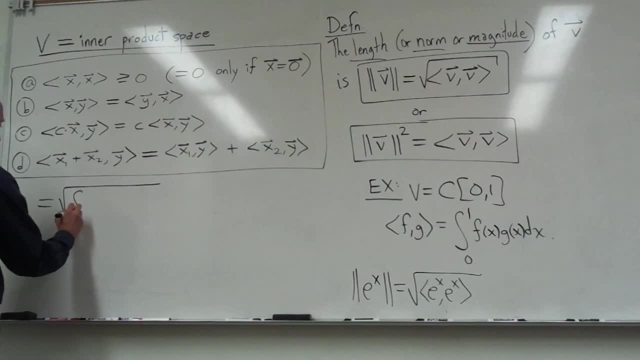 So this is the square root of well, I'm going to be doing the integration from zero to one right of e to the x times, e to the x. Well, e to the x times e to the x is just e to the 2x. 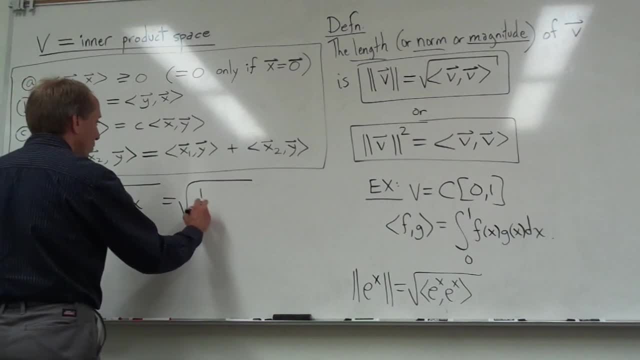 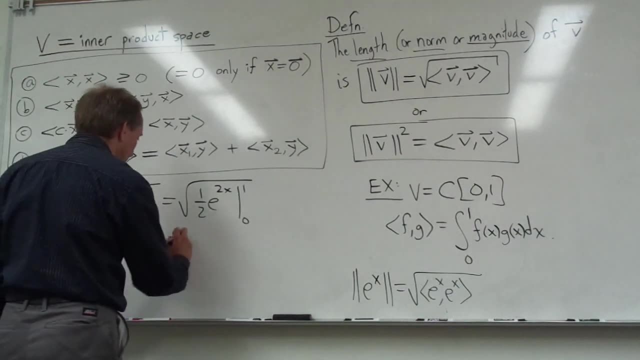 When I integrate that underneath this radical, I get one half of e to the 2x which I now have to evaluate from zero to one. So this is going to give me the square root of one half e squared minus. whoops, this is all under the radical. 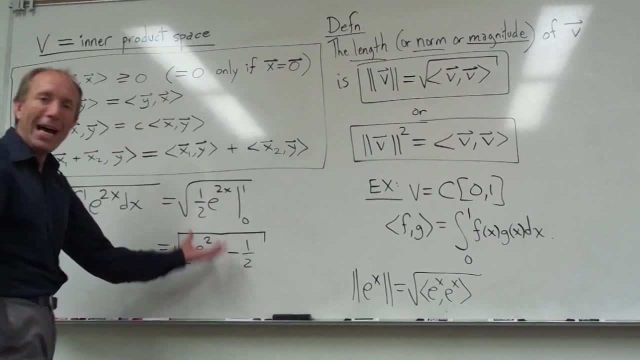 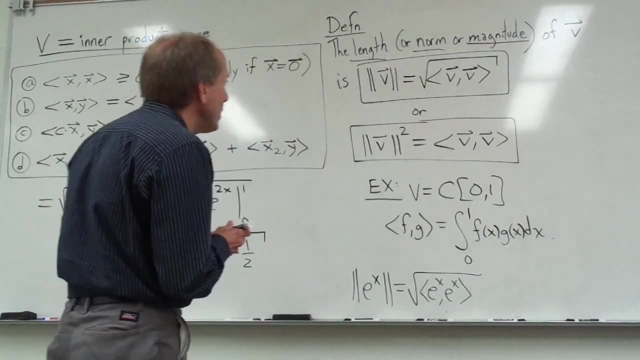 minus one half of one, So it would just be that. Okay, So there's the length, or the norm, of the vector e to the x, right there, Okay. So just to show you a quick example of that. Okay, If I'm going too fast. 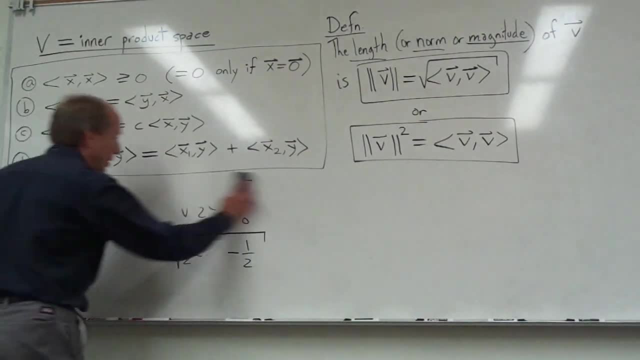 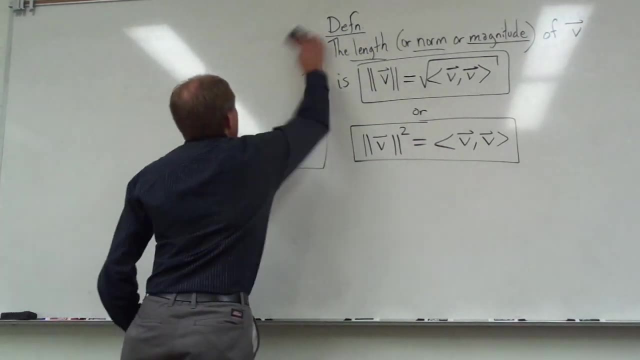 just put me on pause and study what I've got up here. I'm going to move on. Let me actually start up here again, in the top left. So actually let me put one more thing right here. first, If the norm of a vector 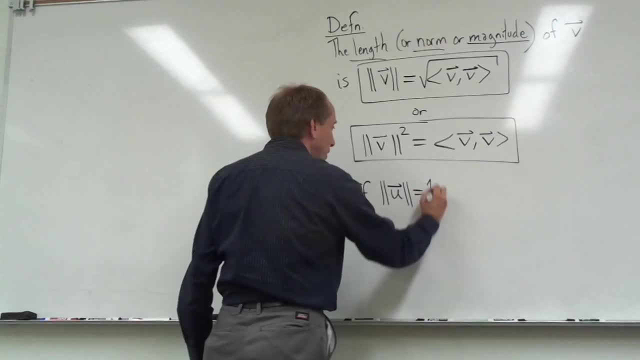 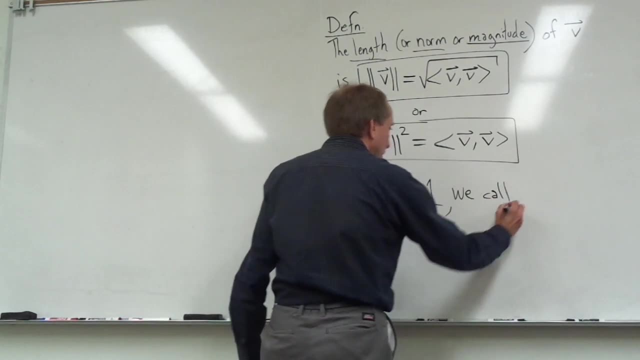 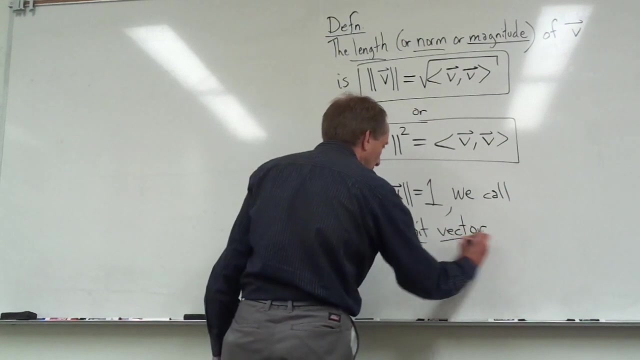 I'm going to call this one u. if it equals one, then we call that a unit vector. Okay, So you've seen these before in other classes, but it's worth recording it here as well. So a unit vector just has length one. 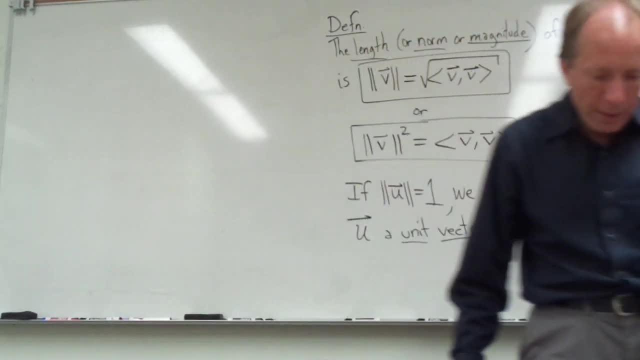 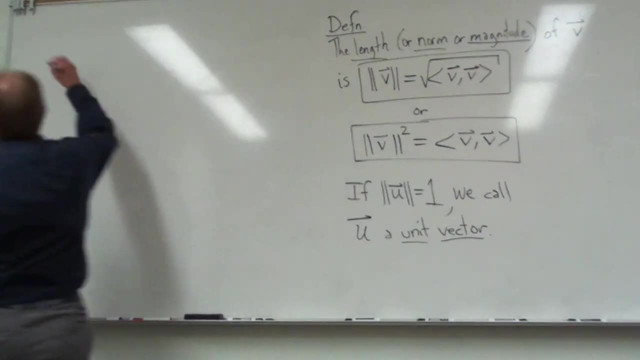 Okay, And sometimes we're going to be favoring unit vectors, you know, over other types of vectors. Okay, Let me just show you a quick little example of something that we can do just with what we've done so far, Okay. 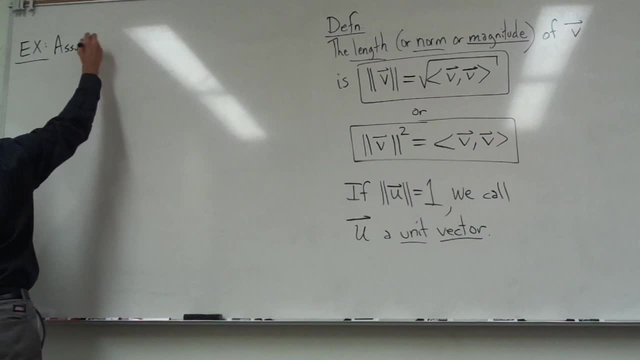 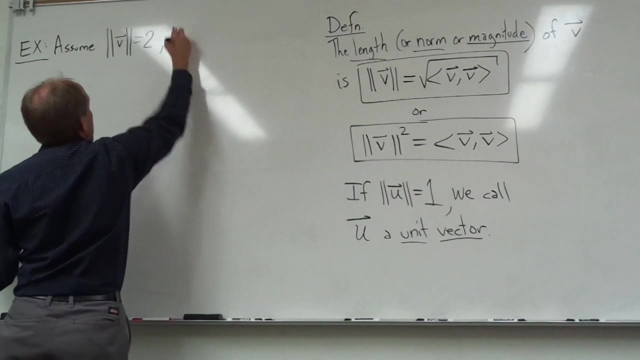 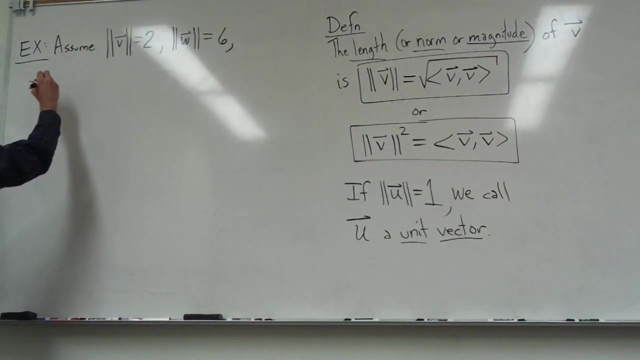 So let's assume I'm not even going to tell you what kind of vectors these are, but let's just assume that I have a vector v whose norm is two and that the norm of the vector w is six and that the inner product of v and w 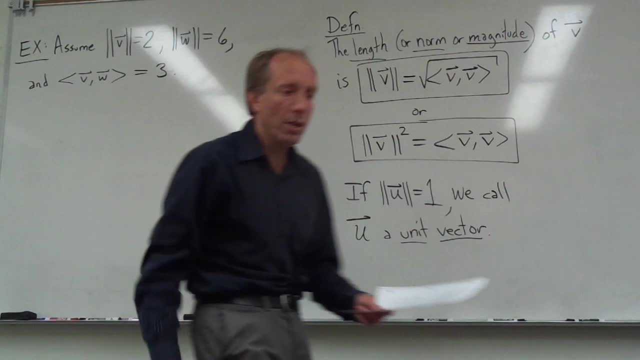 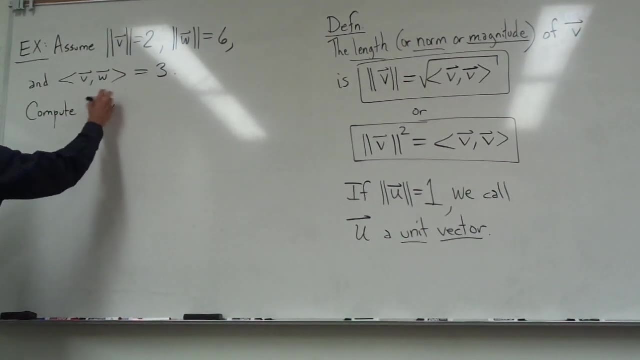 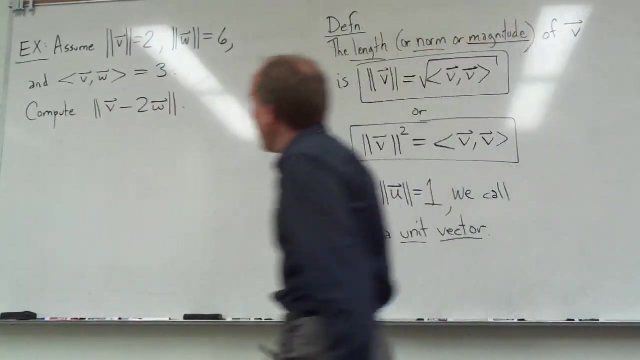 is equal to three. Let's just say we know those values. Okay, Let's try this little problem. Let's compute the norm of v minus two w. All right, See if we can actually calculate that. Okay, Well, we have our formula for the norm. 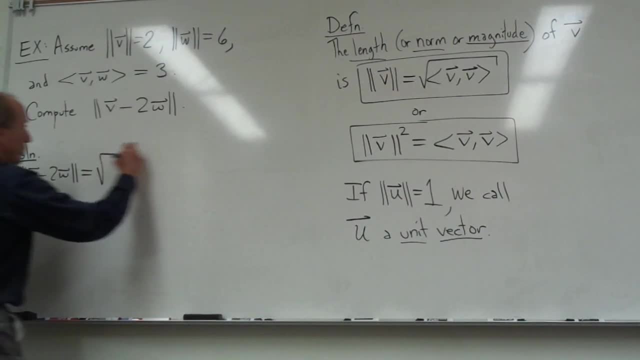 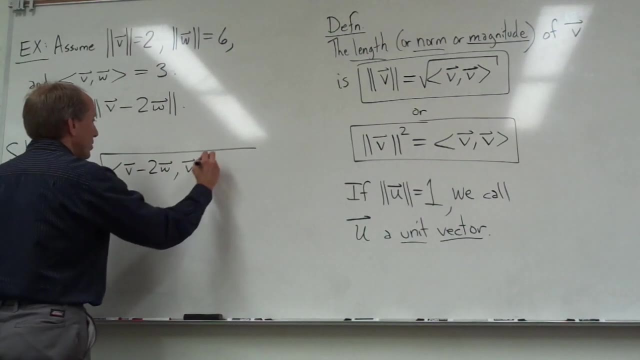 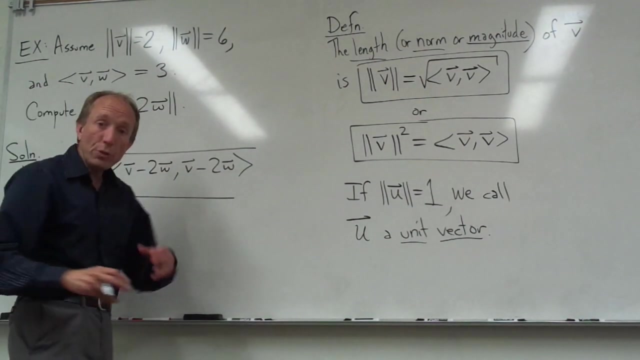 The norm is just the square root right of the inner product of this vector with itself. So I just put that here like that And what I can do is okay, using those inner product axioms, I can essentially FOIL this out right. 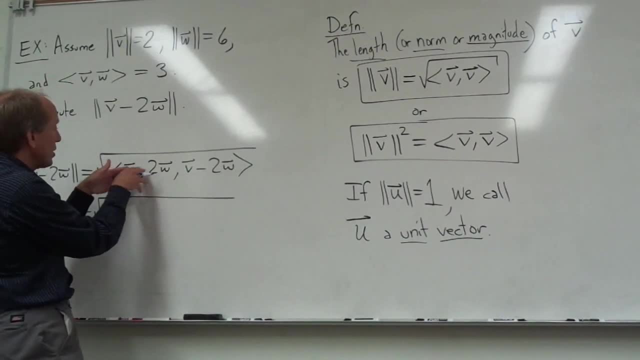 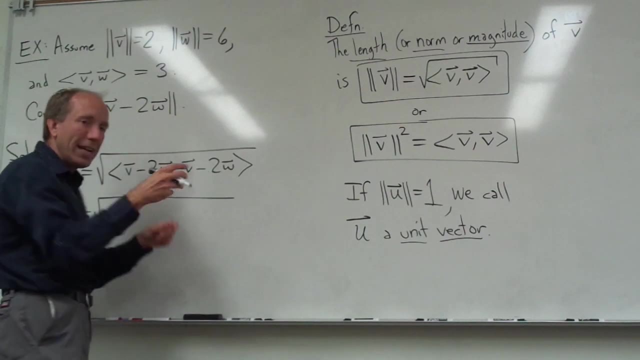 We have the property d that says I can split up plus signs or, in this case, minus signs, And we also have property c that tells me that I can pull those factors of two out. So if I literally just kind of FOIL this apart, 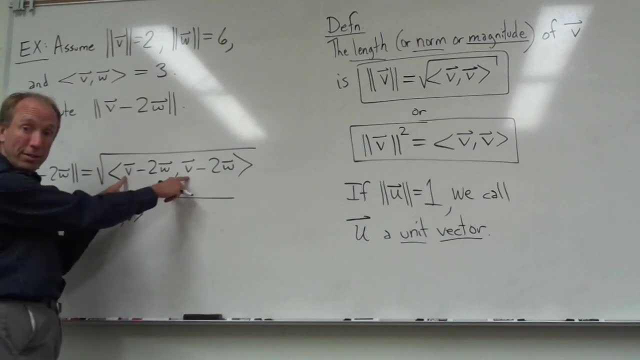 I'm going to get you know. the first term here is the inner product of v with itself. Then I'm going to have a subtraction, I'm going to take out the two and I'm going to put the inner product of v with w. 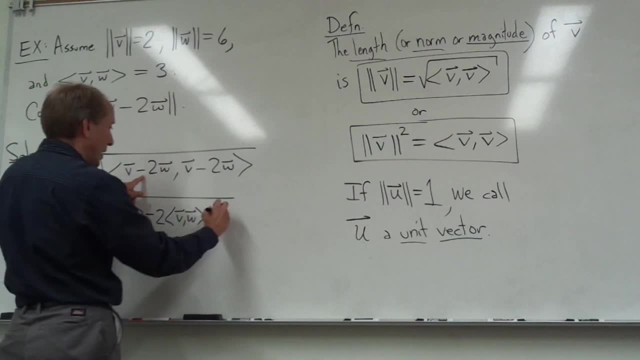 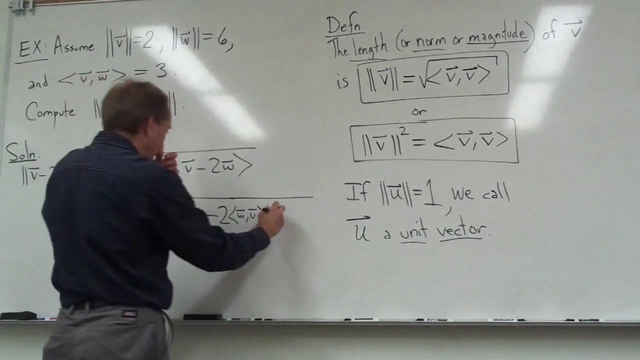 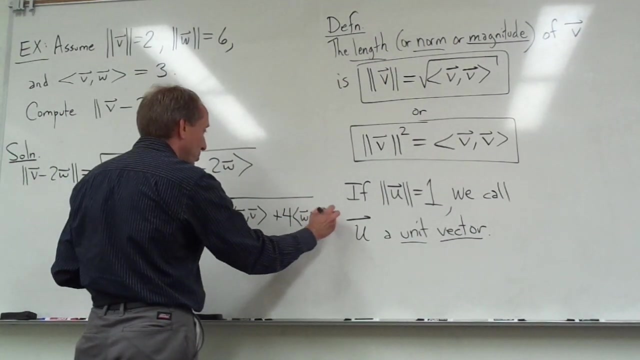 Okay, Then I'm going to FOIL the inner term here. There's another minus sign and there's another two. The inner product of w with v, And then finally the two minus signs, And I have two factors of two, which makes four times the inner product of w with itself. 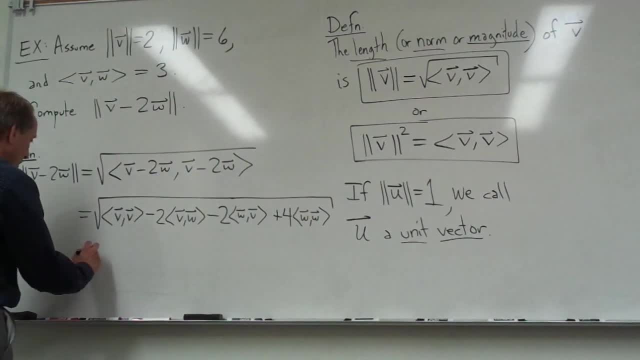 Okay, So it's going to look like that. Now, the first term is just the norm of v, It's squared, right. So the inner product of v with itself is just the norm of v, squared. That's just this formula, right here. 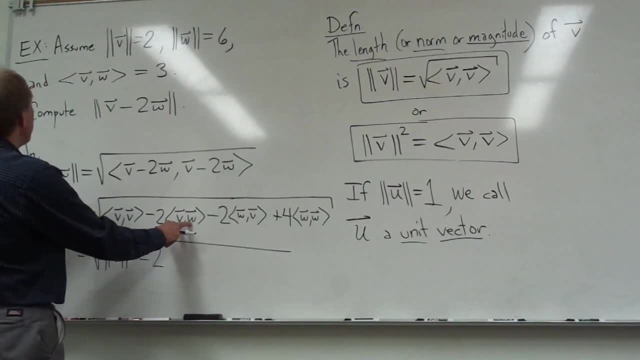 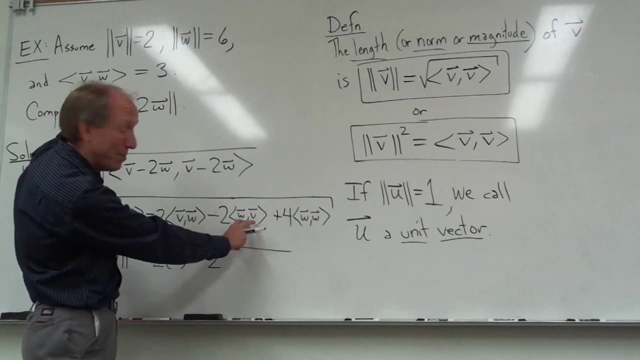 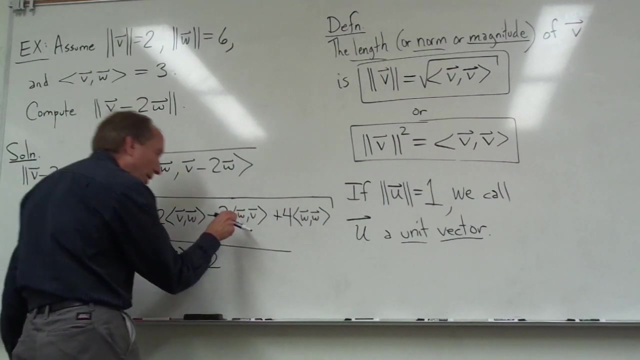 Then I have minus two times the inner product of v with w, which was given as three, And then minus two times the inner product of w with v. But remember that property b of our inner product tells us that this value the inner product of w with v. 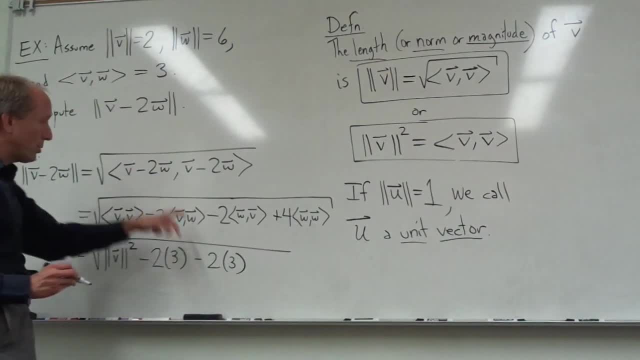 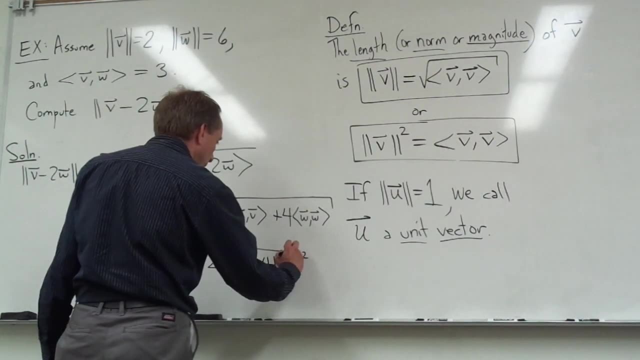 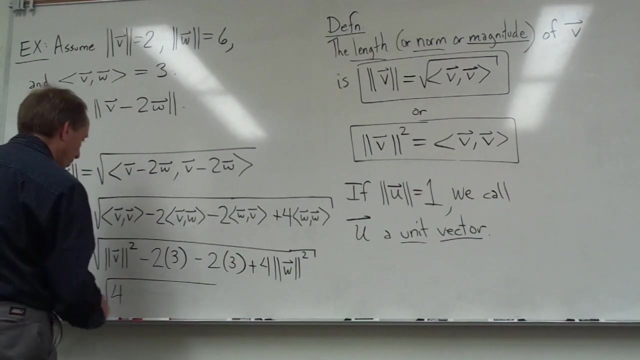 has to agree with the inner product of v with w, So that's actually also three, And then I have plus four times the norm of w squared. Okay, So if I now just plug in all of my numbers and simplify it, the norm of v? squared is four. 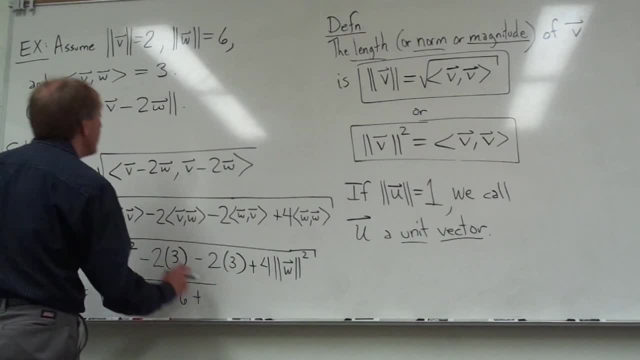 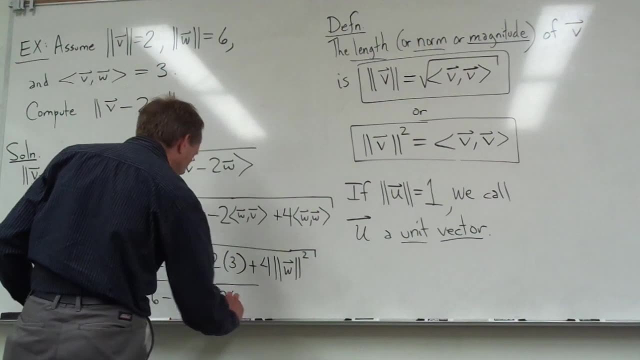 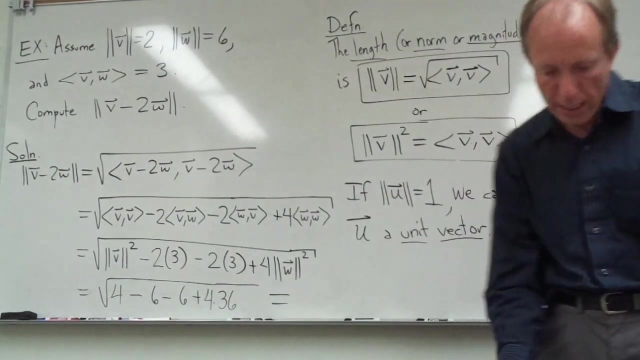 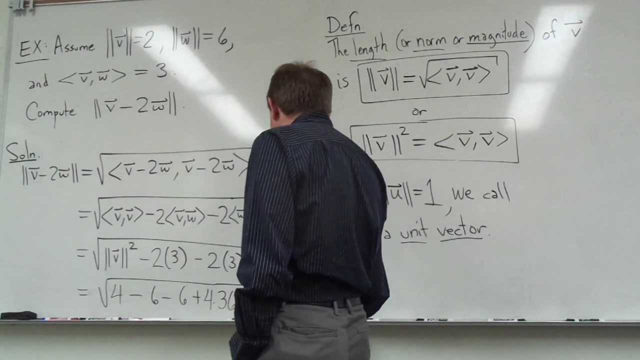 And I have minus six, minus six and then plus four times. what is this going to be? The norm of w squared, which is thirty-six, like that, And so I get some fairly big looking number here. Well, thirty-six times four is a hundred and forty-four. 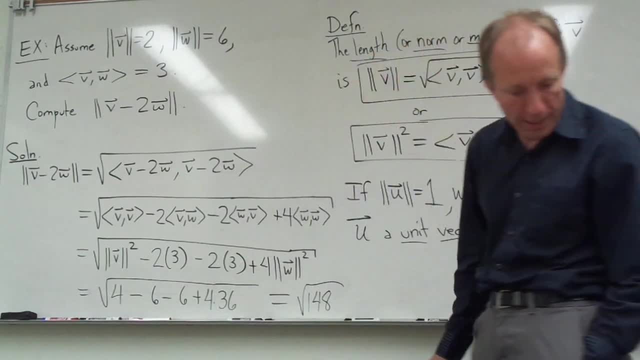 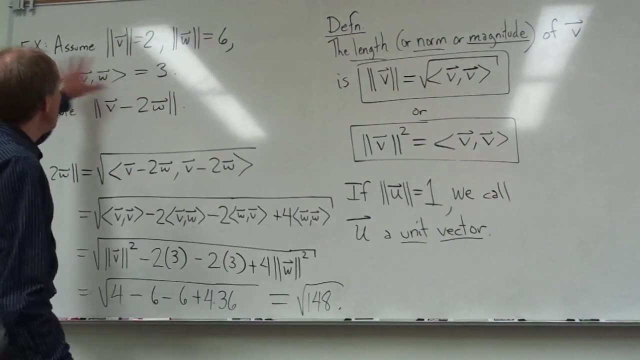 I think it's the square root of a hundred and forty-eight, if I did everything correctly there. Okay, So just a little practice with the, you know, using this given information right together with the axioms of an inner product. 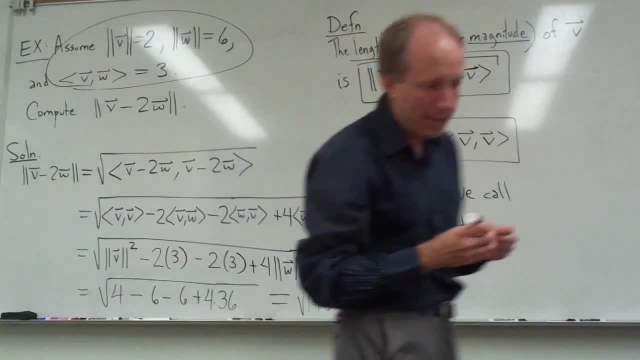 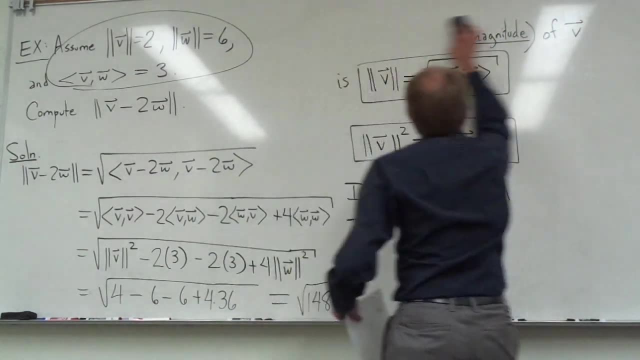 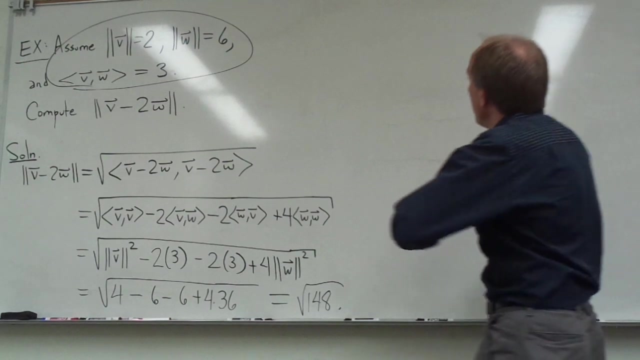 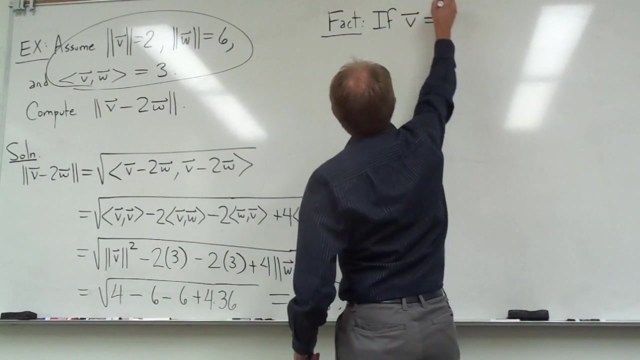 we can actually do this calculation pretty easily. Okay, Let me tell you that. okay, so another little fact here is that you can take any vector at all and turn it into a unit vector. So just a little fact. Okay, So if v is not zero, 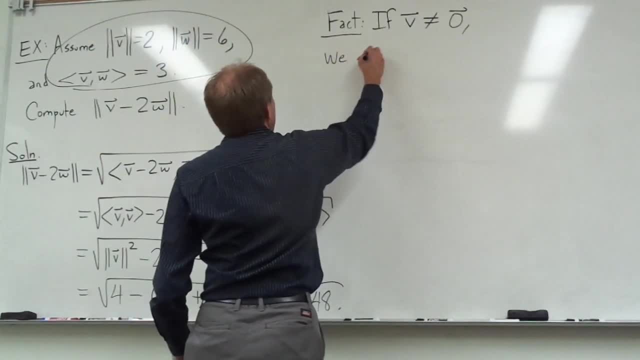 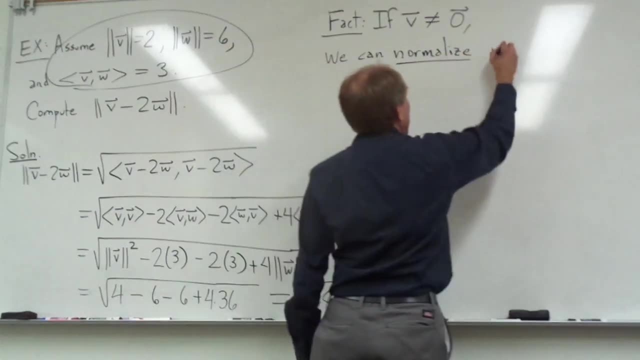 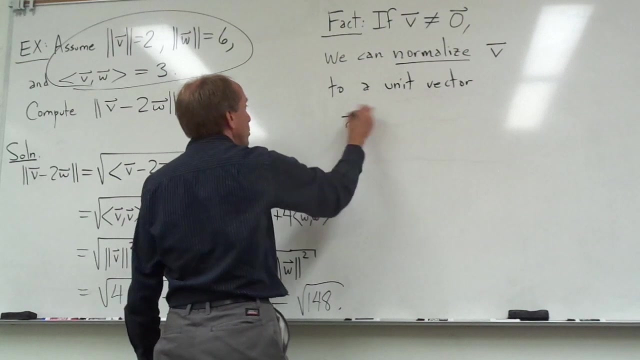 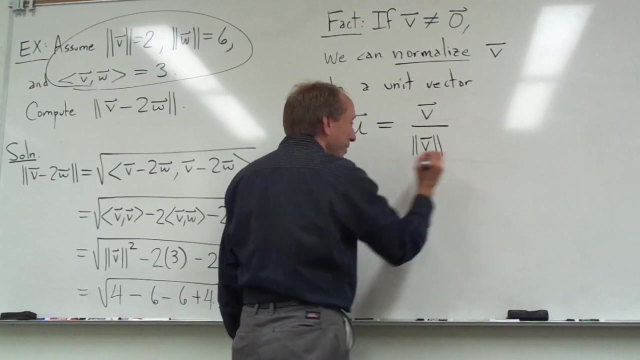 as long as you don't have the zero vector, we can normalize. it's called the normalization process. we can normalize v to a unit vector And I will call that u. and the way you do it is: you just take v and you just divide it by its norm. 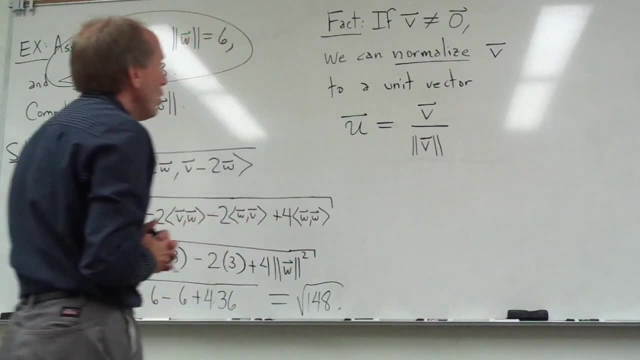 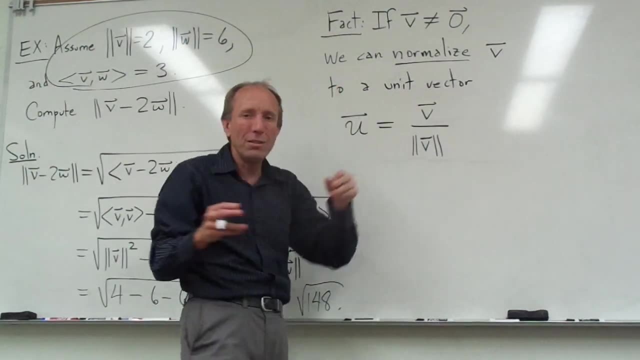 which will be some positive number, right. So turns out that what you're doing is you're shrinking the vector v down so that it essentially still- you know- has a lot of the same properties that v does. So it might be, you know. 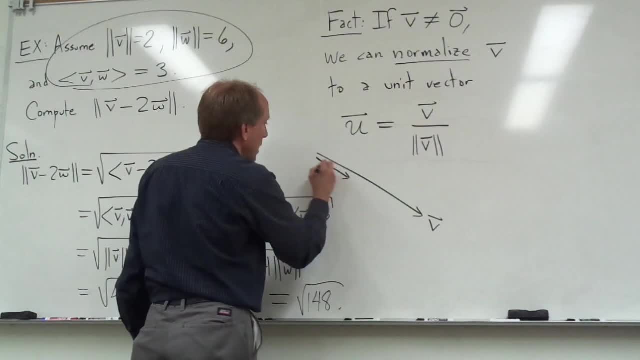 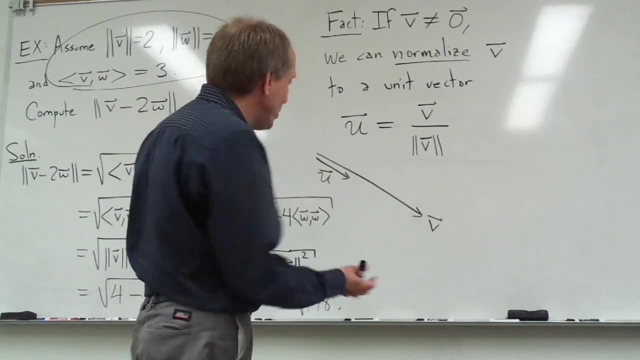 if you think of it visually, there's v. The vector u is kind of just a compressed version of v that's been reduced to a length or a norm or a magnitude of one. Okay, So this is an easy, an easy thing for us to do. 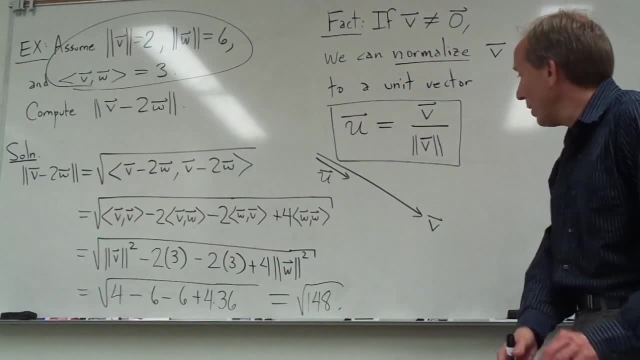 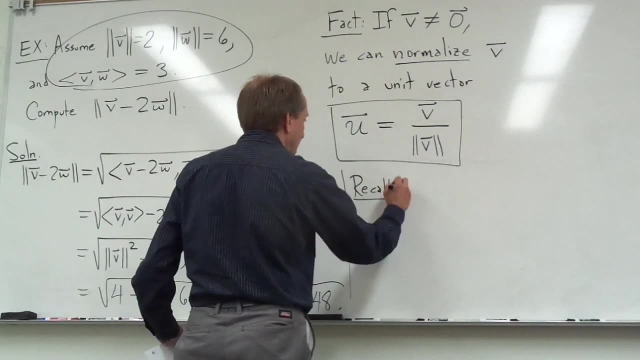 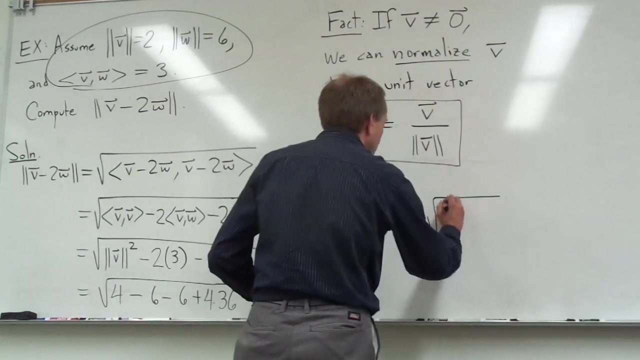 We can normalize any vector in that manner. So, on that previous example where I did so, just to recall, on that last example, I had the norm of e to the x right And my answer was, if you remember, the square root of one half, e squared minus one half. 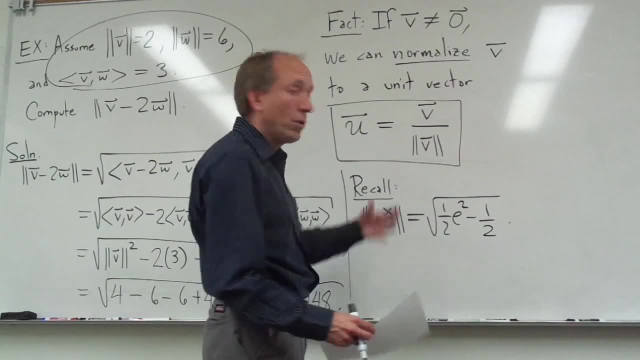 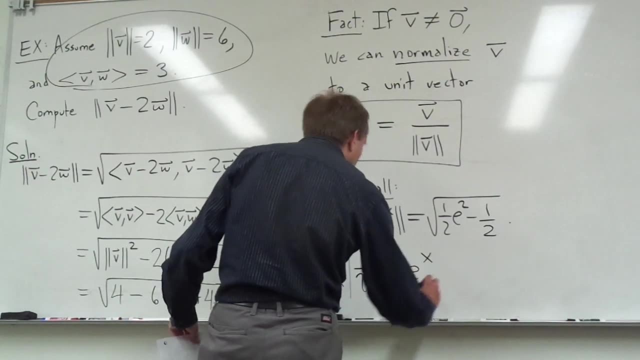 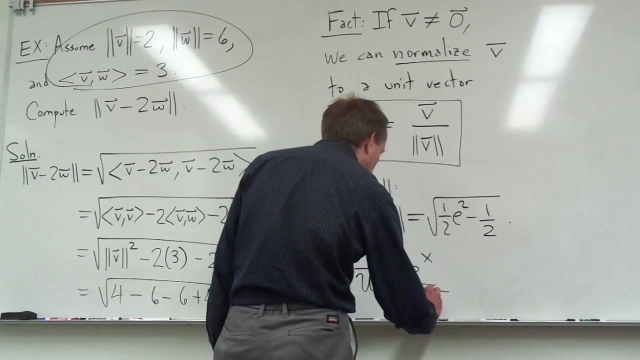 So if I wanted to, I could normalize that okay, and I could create a unit vector which would be e to the x divided by the norm of e to the x, So in other words, divided by the square root of x, So the square root of one half e squared minus one half. 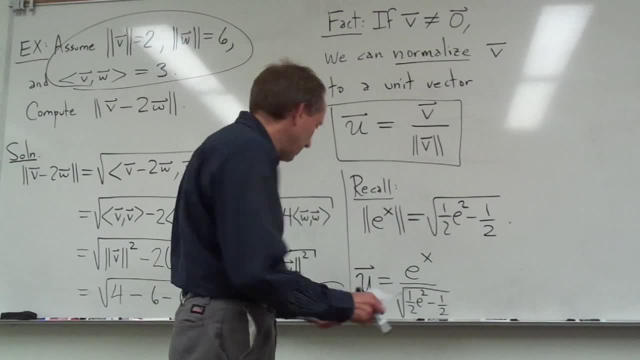 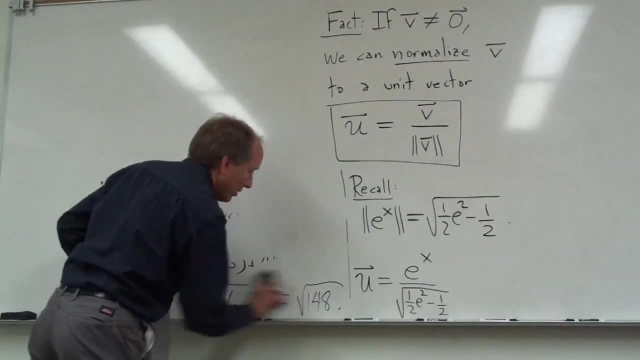 Okay, So you could, you can always do- do those kinds of things. Okay, Let me tell you about the angle between two vectors. Okay, Hope everybody's hanging in there. This isn't going to be too much longer. I just want to get a couple more definitions up here. 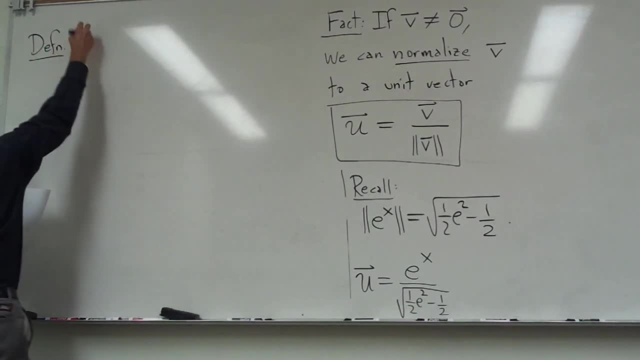 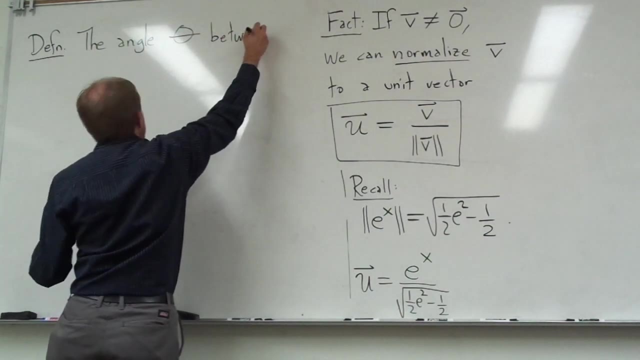 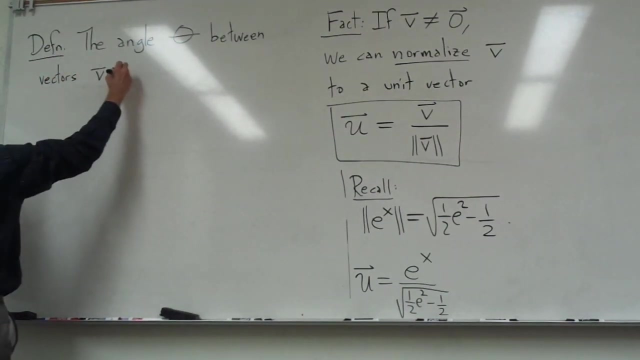 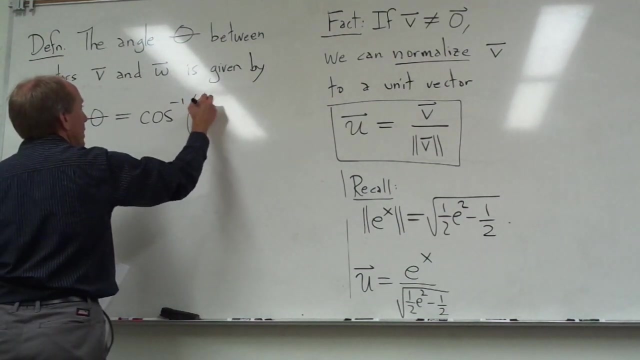 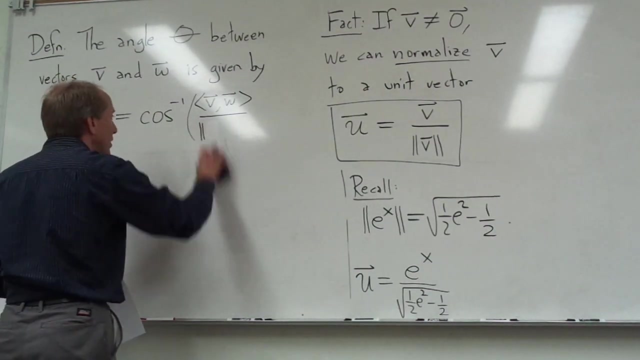 Okay, So a quick definition. The angle theta between vectors v and w is given by. so here's the formula. This is the definition. right, It's the arc cosine of the inner product of v, with w right divided by the norm of v. 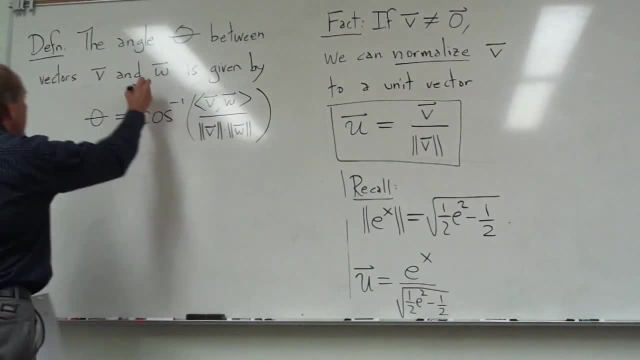 times the norm of w. Okay, So this is an important equation right here. Or in other words, the cosine of theta is equal to- I'm sorry, let me write the formula a little bit differently- The norm- sorry- the inner product of v with w right. 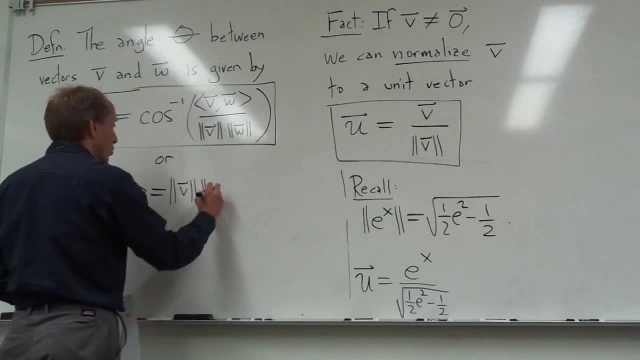 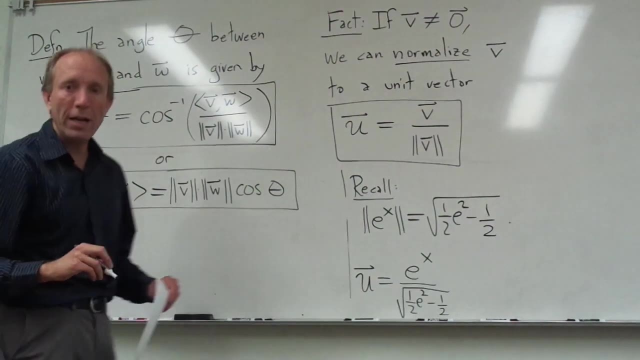 if I solve for that, it's just the norm of v times the norm of w times the cosine of theta. This is a better way to write it And this should look familiar from your multivariable calculus class right. This is another dot product formula. 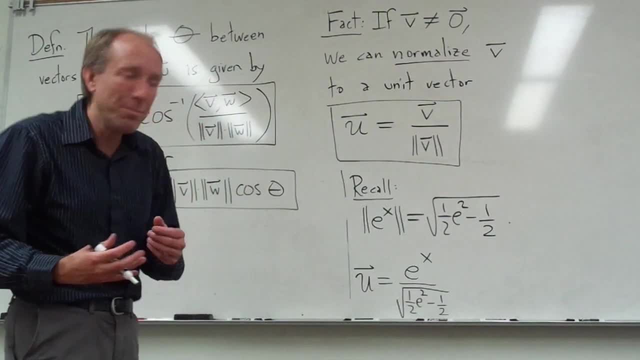 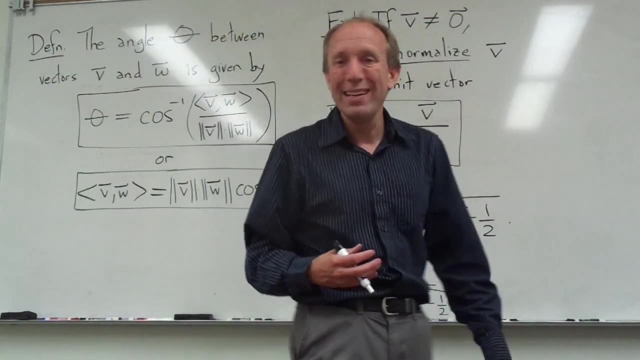 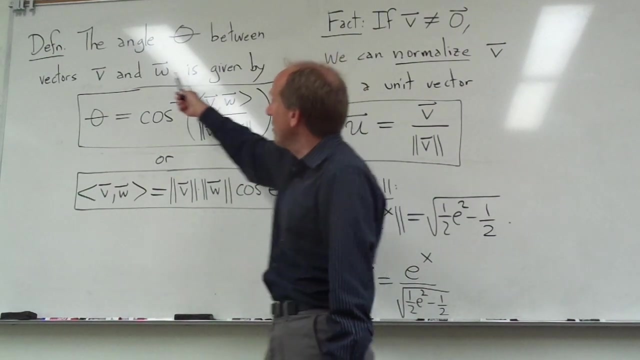 We're just using that dot product formula from multivariable calculus to define an angle in the context of any inner product space. So we should be able to calculate the inner product of two vectors. find their norms okay, I'm kind of depending on the vectors being non-zero here. 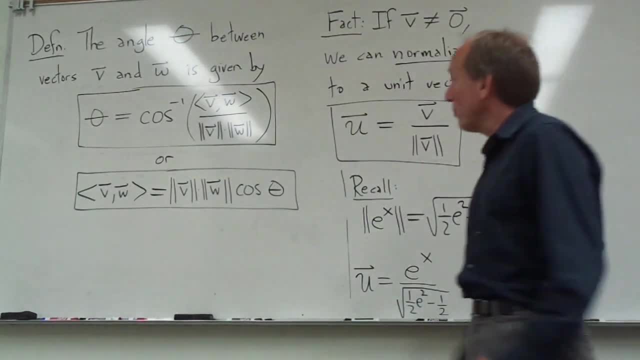 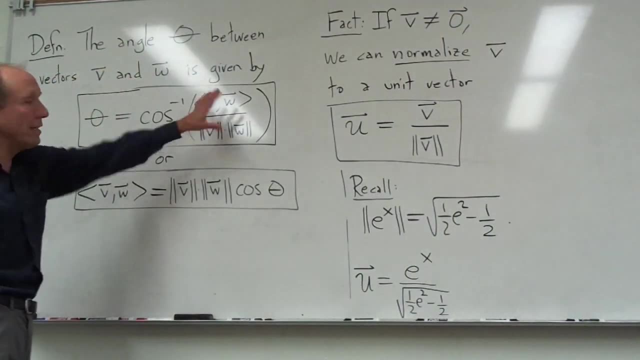 otherwise this isn't particularly interesting. But we can certainly calculate this, you know, by just calculating the expressions that you see in the parentheses there. Now you might be a little bit nervous because you can't take the arc cosine of a number that's bigger than one. 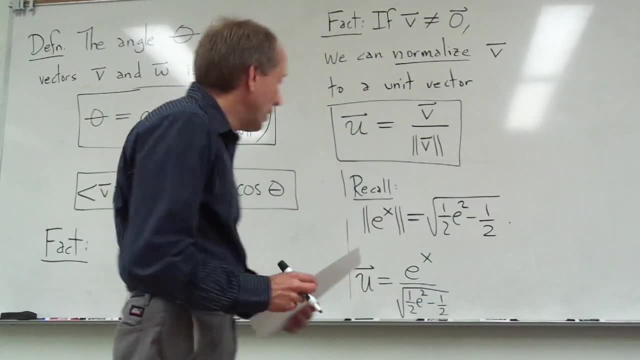 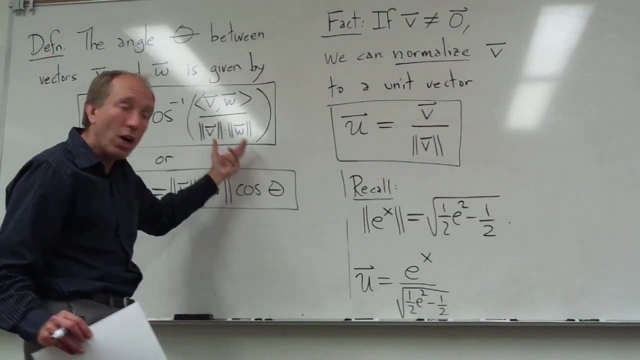 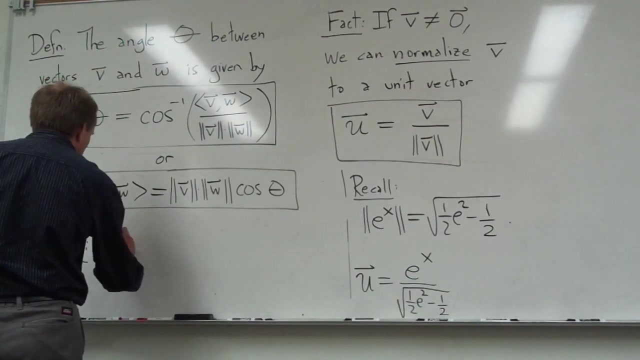 or smaller than negative one. But fortunately it turns out that in this fraction right here the denominator is always at least as big as the numerator. So in other words, the absolute value of the inner product of v with w is always at most. 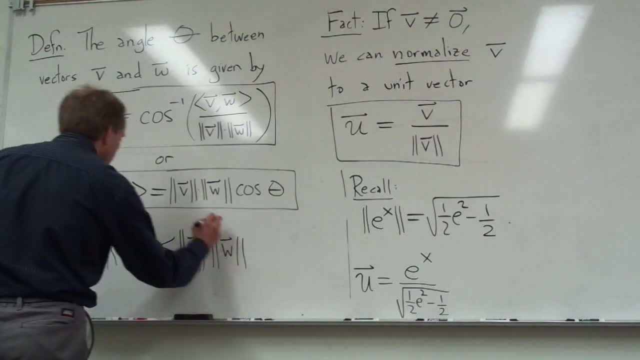 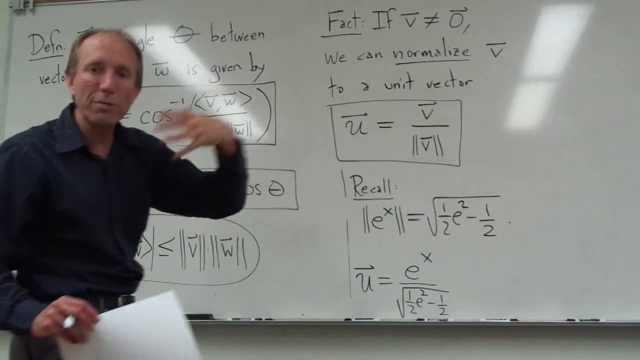 we're not going to need this fact very much. this is not really something that you need to worry about too much, but I just want to make the point here that this arc cosine function really is going to make sense, because what you've got is: 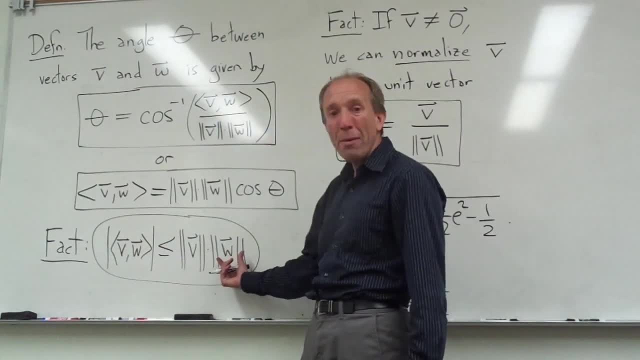 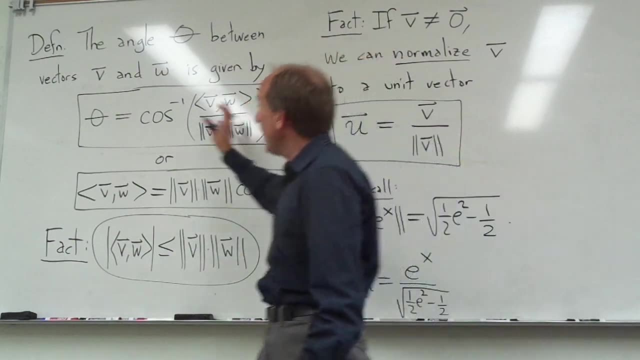 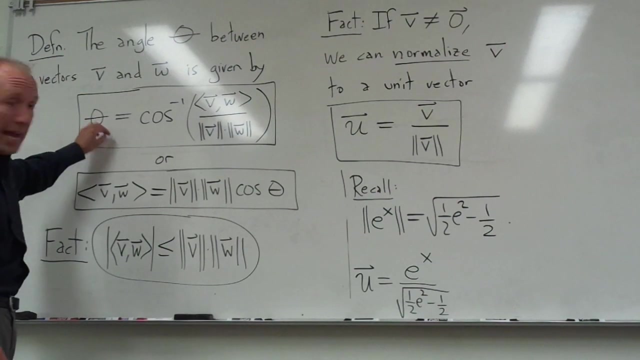 you've got a numerator that is smaller than the denominator, So the fraction is less than one. in particular, it's between minus one and one, and I can take the arc cosine of that and come up with theta. okay, Obviously, the actual angle. 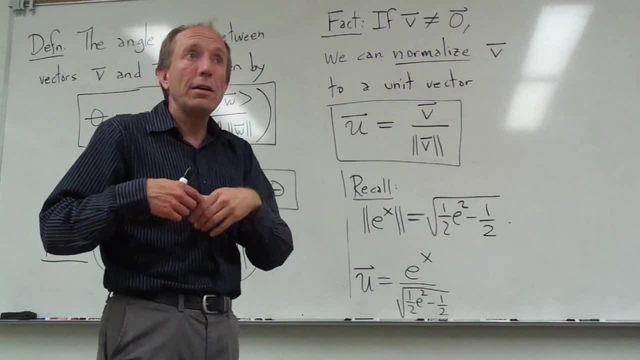 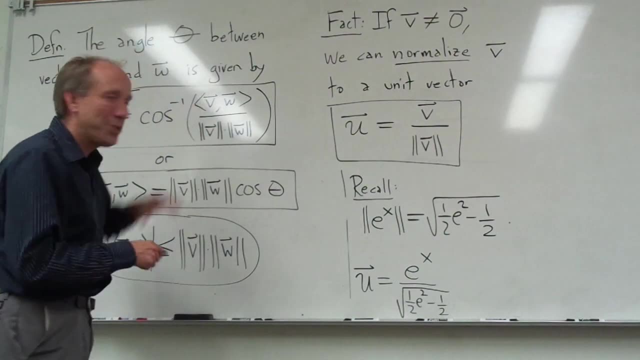 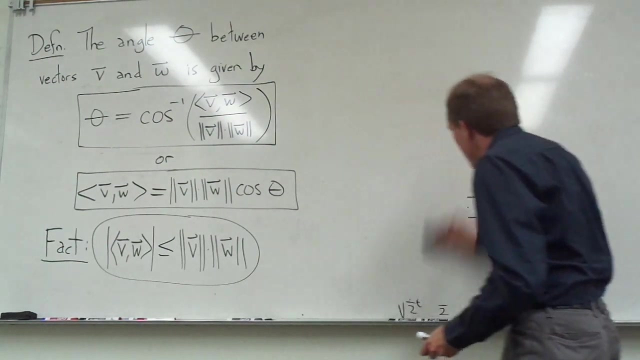 is going to depend on what my inner product formula is right. Remember, we have to be given an inner product in order to do all these calculations here. So you know the answer that you get for theta is going to change if you change your inner product, right. 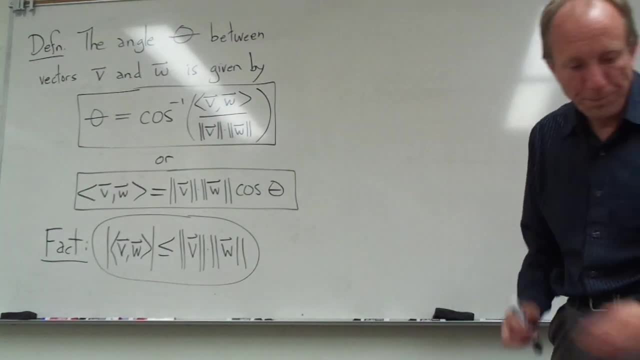 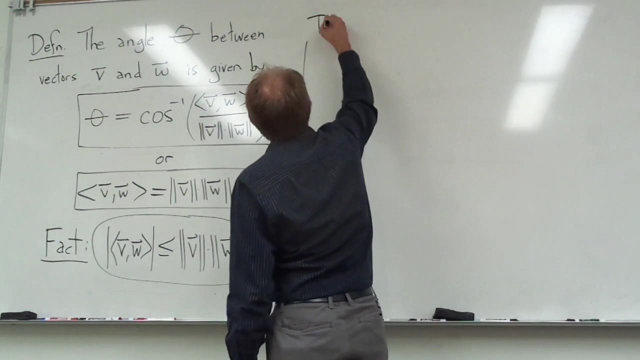 So that's just something else to keep in mind. From this information here, you know we can already prove little things like, so I'll show you, for example, something that you've probably known for quite a long time, which we can now show is true. 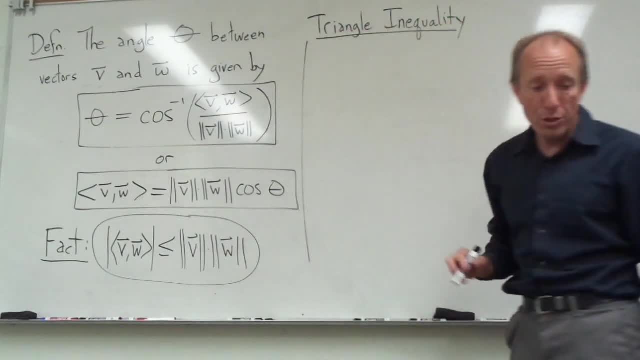 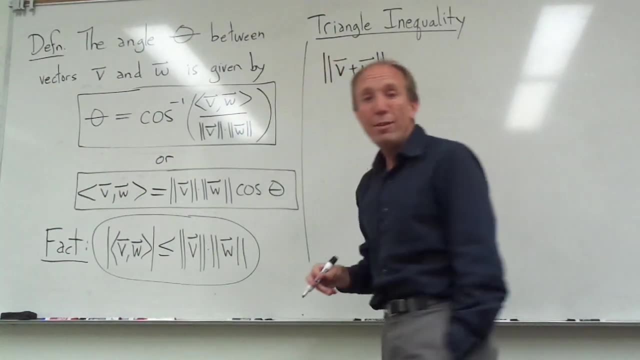 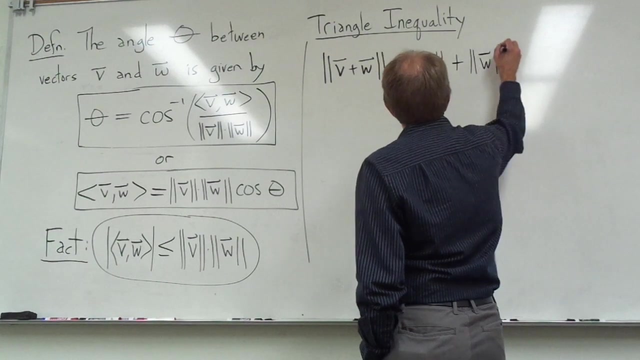 in any inner product, It's the inner product space, which is the triangle inequality. All that says is that the norm of the sum of two vectors, okay, is less than or equal to the sum of the norms. Okay, so this is a nice little property. 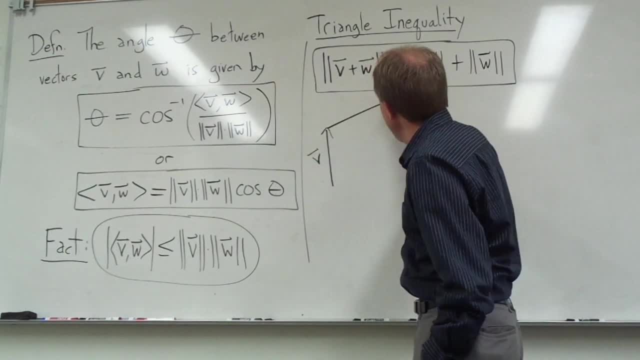 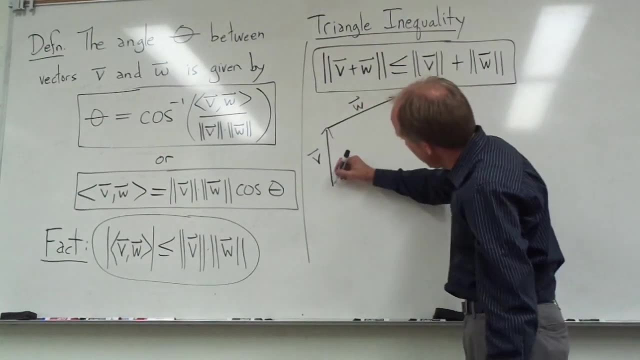 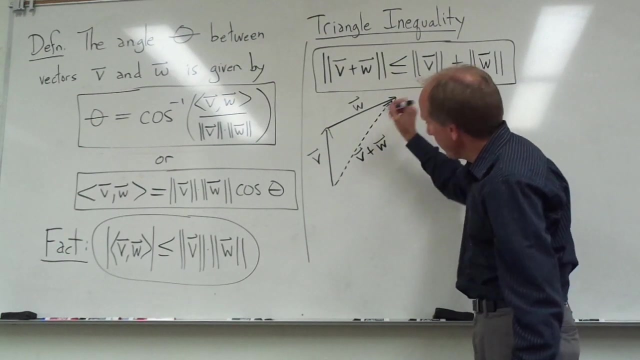 From a geometry point of view, if you think of the vectors as being vectors you can draw, if I put my v and my w together, like that, v plus w is just the result of adding the vectors, sort of head to tail, like I've shown you here. 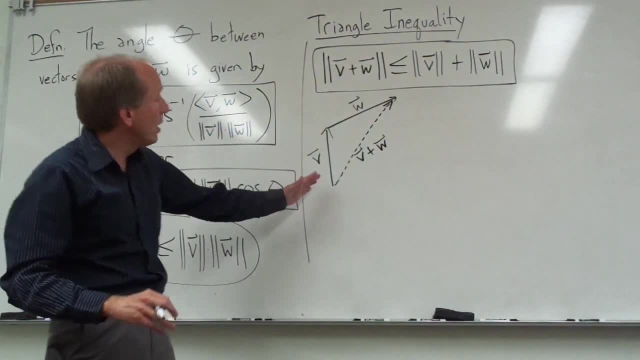 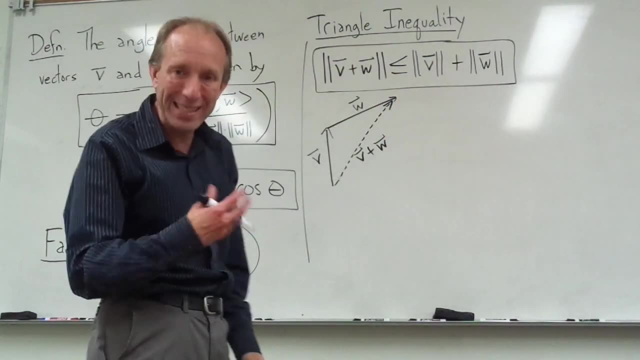 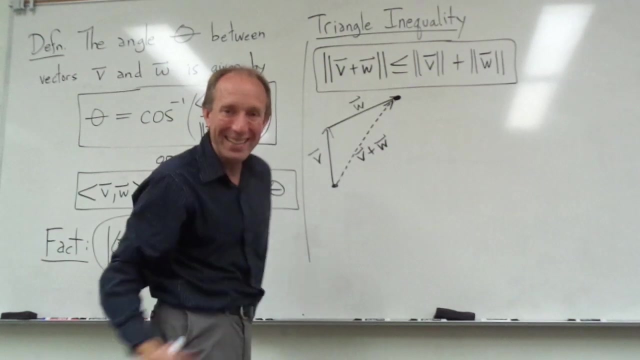 And all that this inequality is saying is that the length of the dotted vector v plus w is less than or equal to the length of v plus the length of w, The shortest distance between two points, these two points, is a straight line, okay. 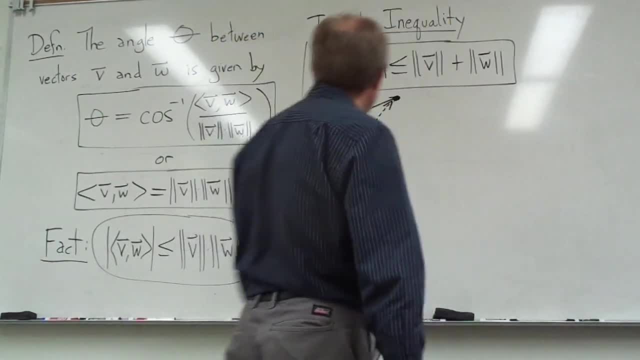 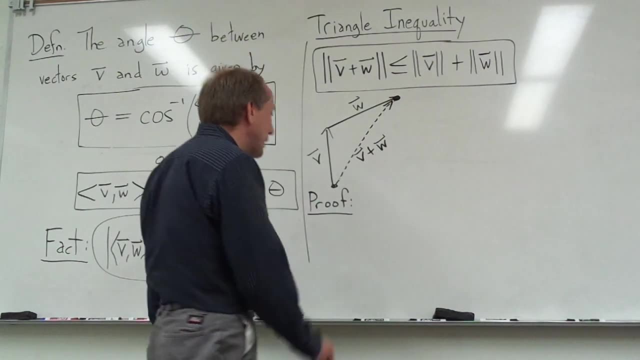 Something that we've known, obviously, for a long time. It's kind of neat to just see the proof. You know I don't want to be super proof heavy in this section, but just to show you how we can again. 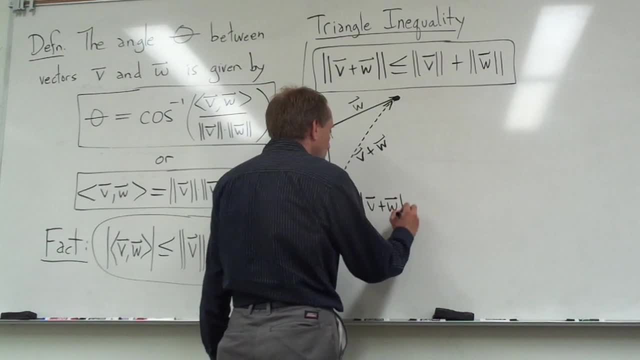 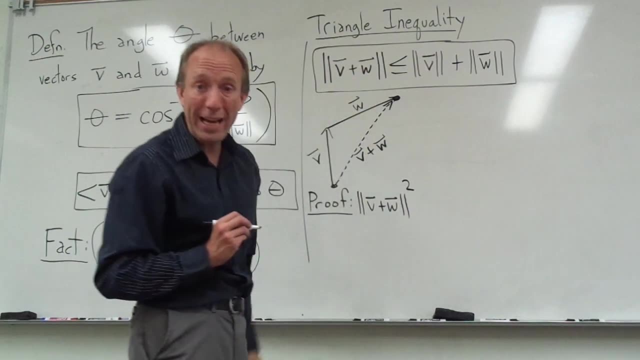 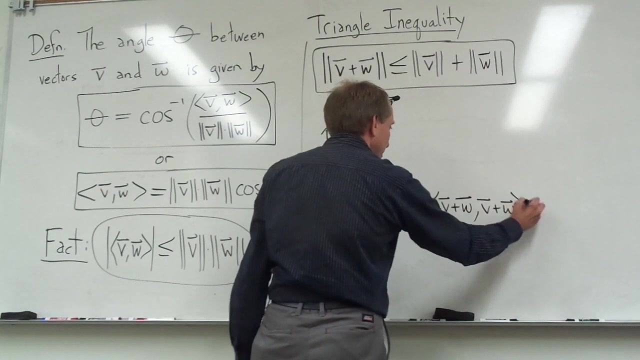 kind of use some of our inner product properties. what I'm going to do is just show you how to justify this right. If I square the left side right, you know that that's just the inner product of v plus w with itself, okay. 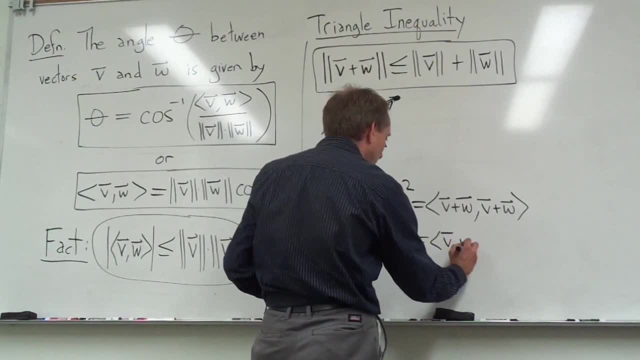 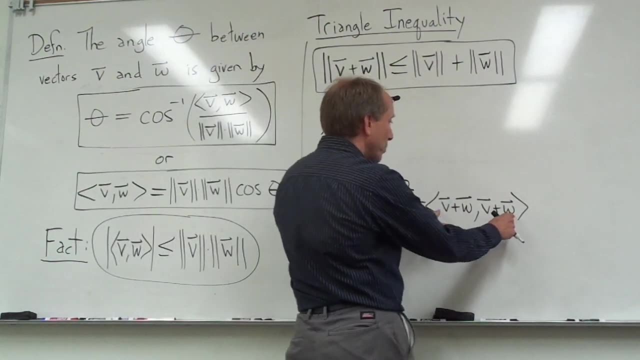 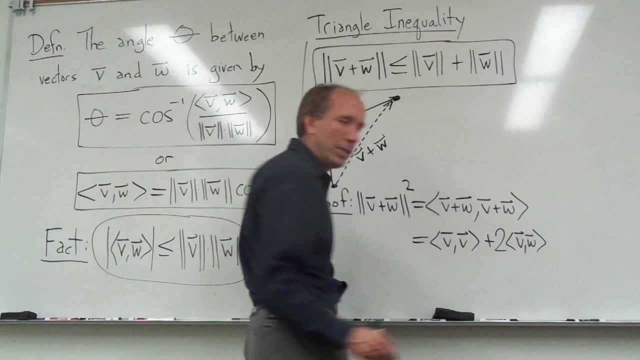 And I can again foil that out, just like I did on that earlier example: I get the inner product of v with itself. I get the inner product of v with w and also the inner product of w with v. So that's two times the inner product of v with w. 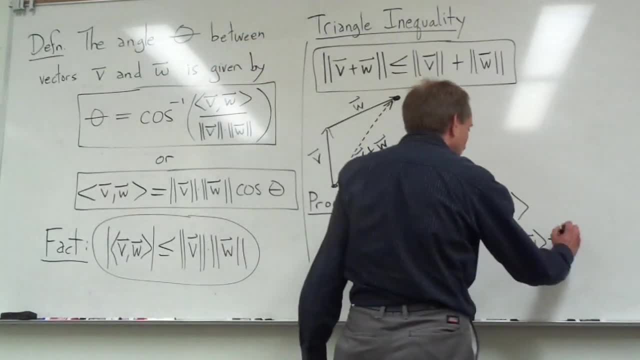 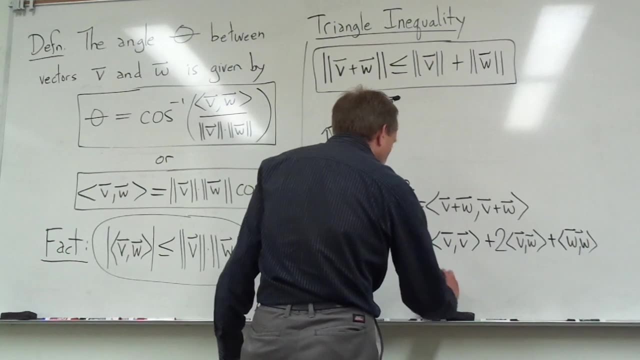 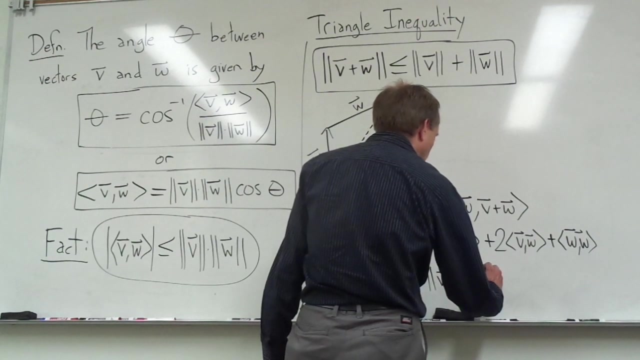 because, remember, they're the same right, Those middle terms are the same. And then I get the inner product of w with itself at the end. So that's just, you know the norm of v squared plus two times the inner product of v with w. 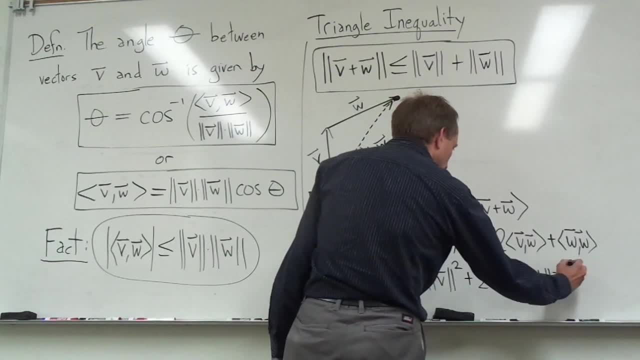 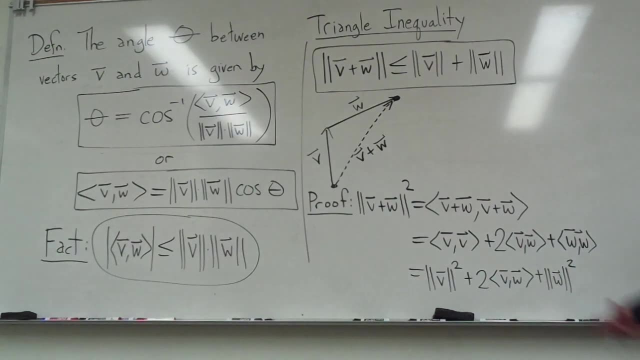 plus the norm of w squared, So we can sort of foil it out like that. And now, if I just use the fact that's over here on the bottom left, right, I can change this to an inequality and I can put in: okay. 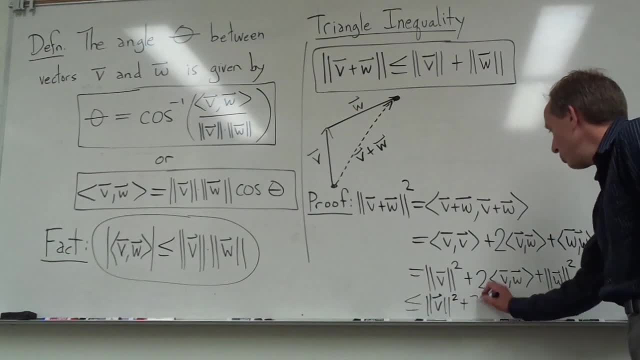 the norm of v squared plus two times the norm of v times the norm of w plus the norm of w squared right. I can just put that in there And that last expression- I'm just going to finish it right here. that last expression is just: 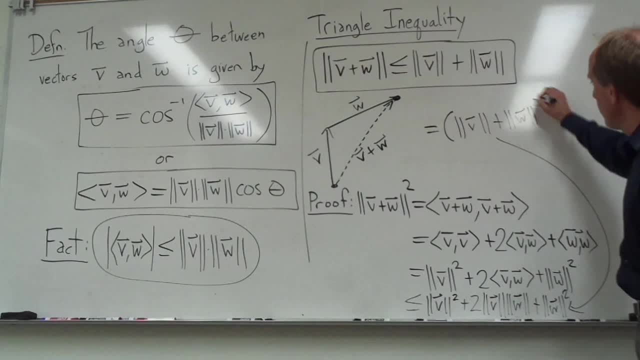 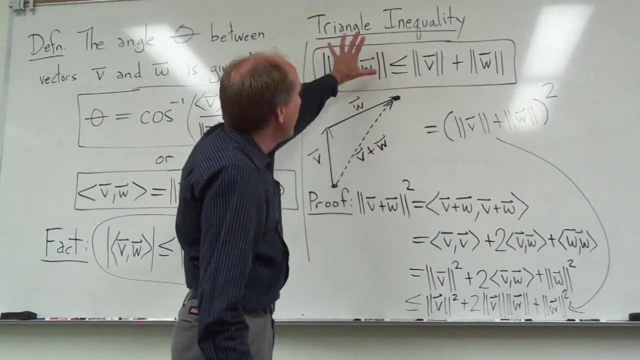 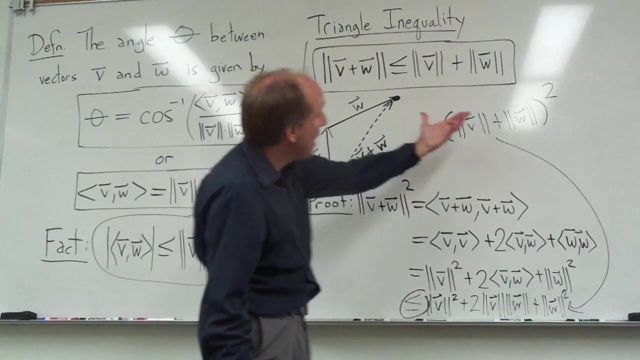 the norm of v plus the norm of w, quantity squared right, And so the square of the left side is less than or equal to- here's my less than- or equal to right here in the middle of this chain, it's less than or equal to the square. 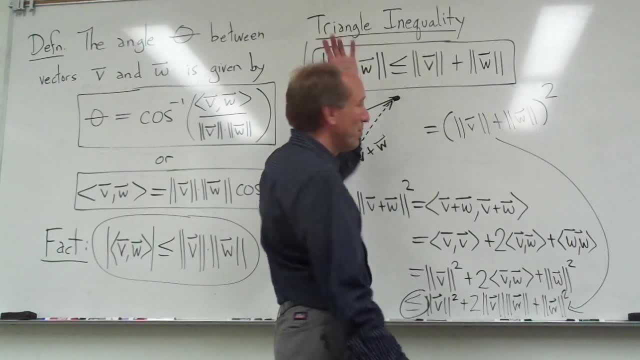 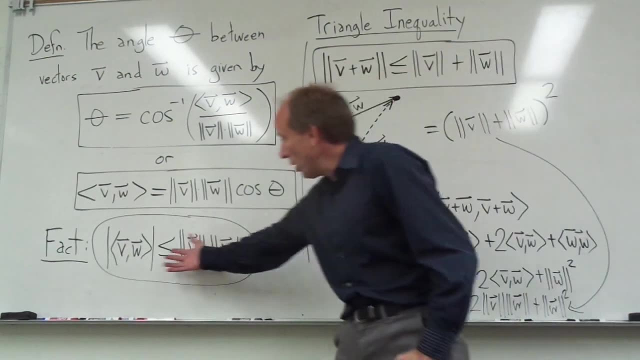 of the right side. So if I just take the square root of both sides, I get my triangle inequality. So that's kind of neat. We can actually use this inequality here. I didn't justify this one. This one is more of a more advanced class. 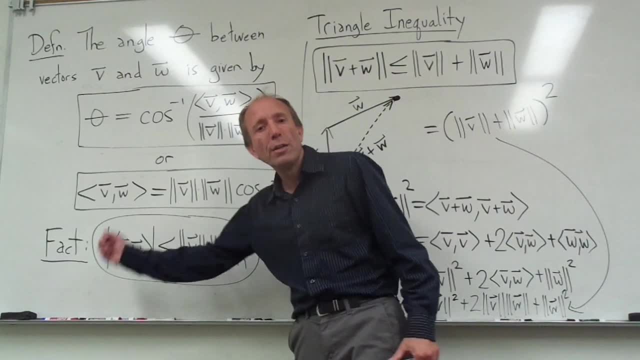 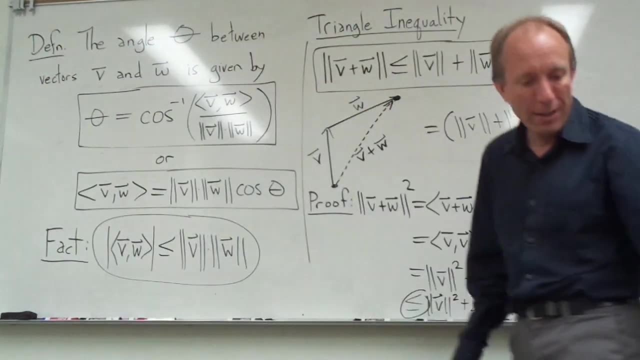 on inner product spaces It's not that bad, but I'm not going to go into it here. But from that fact we can then, you know, show something like the triangle inequality here. Obviously, one last comment here, and then I'll call it good. 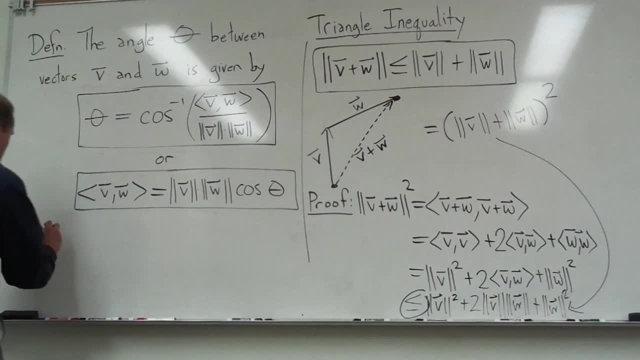 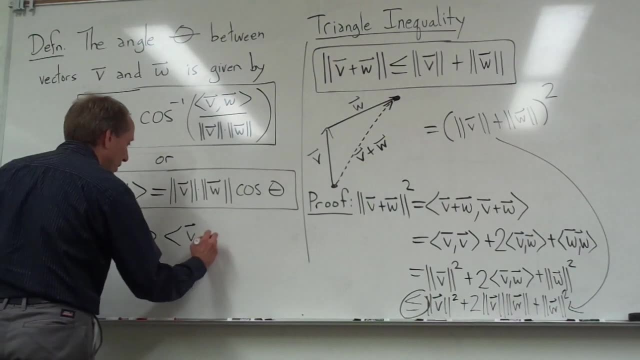 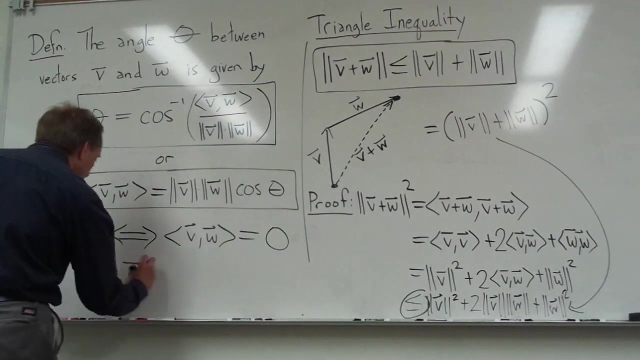 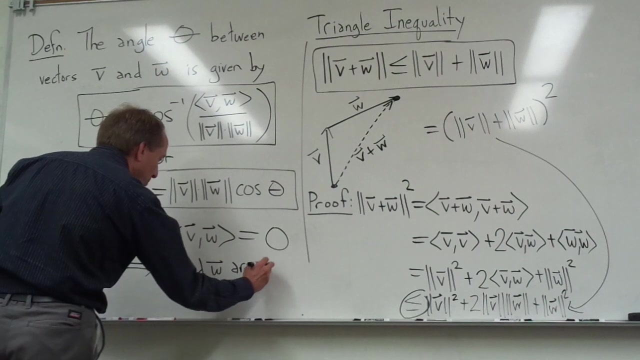 If theta is 90 degrees, right, so theta equals 90 degrees. of course, that means that the inner product of v and w is going to come out as zero. Okay, And that also just means that v and w are orthogonal, They're perpendicular. 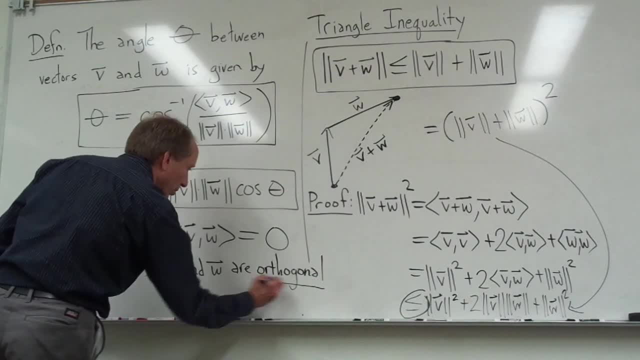 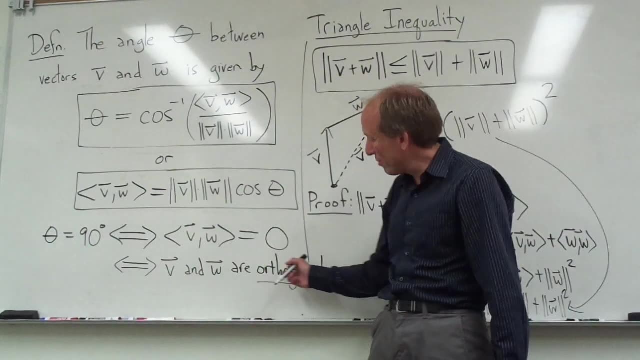 If they make a right angle, a 90 degree angle. they are called orthogonal vectors. They are orthogonal to each other. So a great way to test if two vectors are orthogonal is to just compute their inner product and see if you get zero. 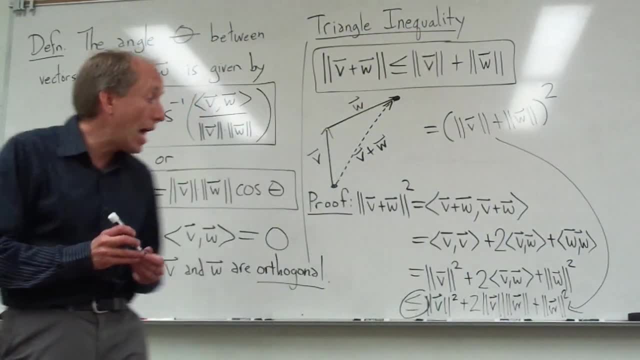 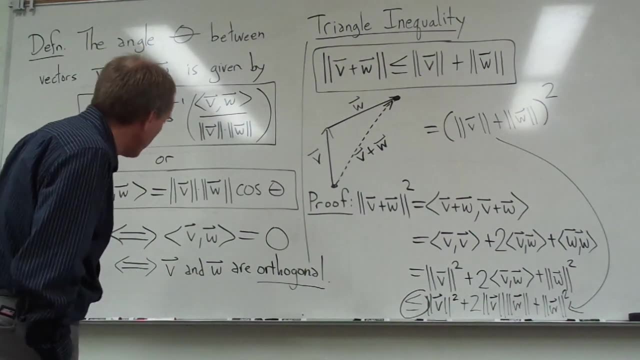 Okay, So just one last definition. We're going to talk about a lot more next time we get together about orthogonal sets of vectors, And so I won't go into it anymore right here. Just wanted to give you a little bit more of that basic background information. 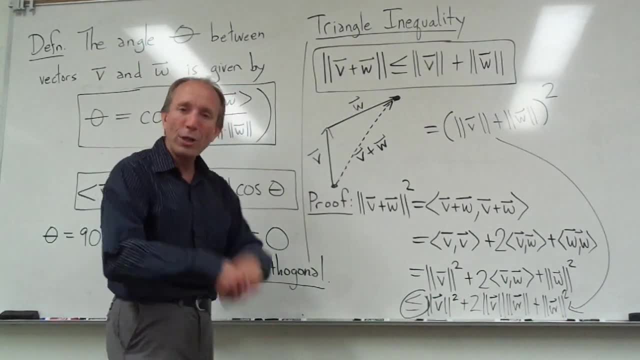 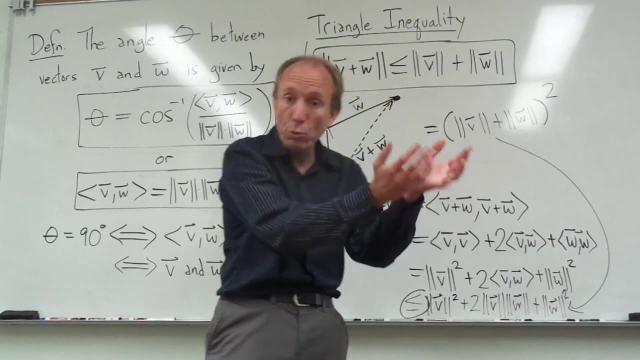 on inner products, inner product spaces. Keep working with the axioms. Make sure you learn them, Practice them. Look at examples of things that do work as inner products, things that don't work as inner products and some of the computational problems. 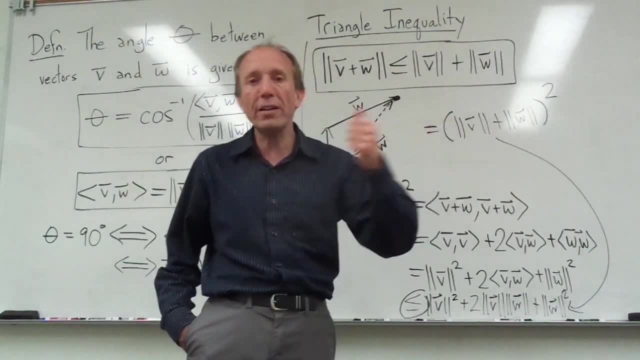 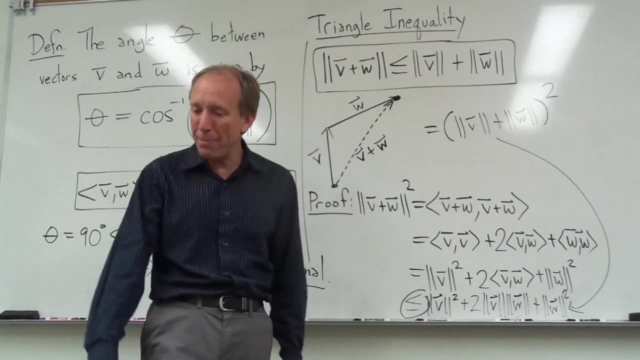 that you can do, Be able to find norms of vectors, angles between vectors and so on. Hope this was useful. I'll be happy to answer questions, kind of go over it again in a little bit more detail if we need to do so. 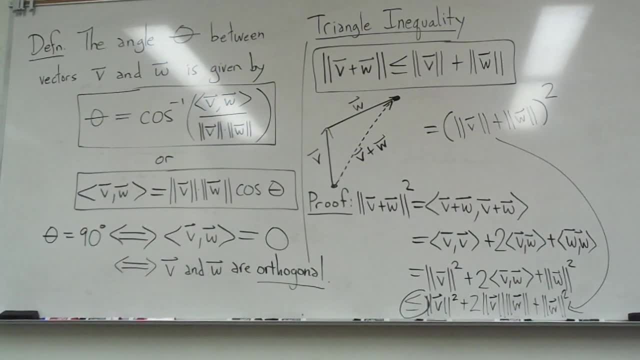 But at least for now, this is a start. Thanks so much for watching, guys. I'll see you soon.